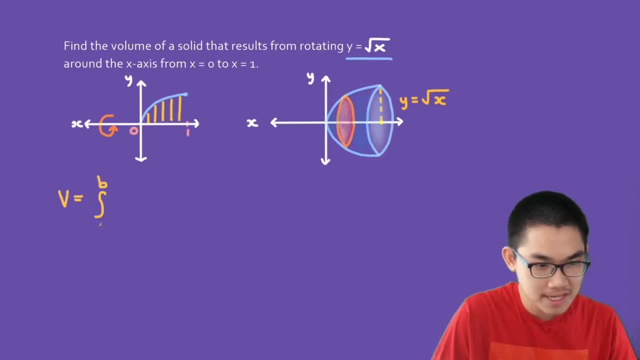 is equal to the integral from a to b of a of x dx where a of x is the area of the cross section. So since the cross section is on the x-axis it is easier to integrate with respect to x. Now let's find the area of this circular cross section. So the area of a circle is the same as pi times the radius squared. This is the same as pi times the radius which is the square root of x to the power of 2 and that will simply be pi times x. Now we successfully found the area function. We can put this back into the integral and that's gonna basically give us the volume of this solid. So let's do that. Now the volume goes from 0 to 1 so that's going to be the integral from 0 to 1 and this is our area formula so pi times x dx and since pi is just a number we can always bring it outside of the integral. 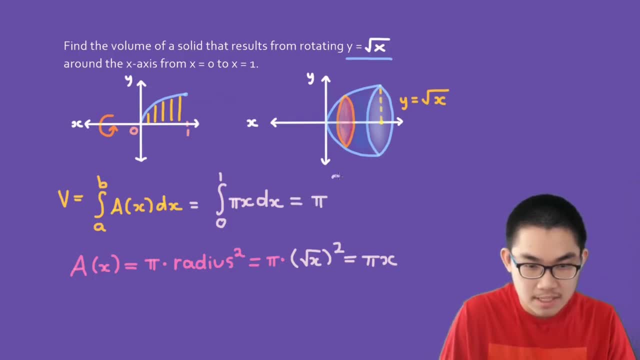 This is the same as pi times the integral from 0 to 1 of x dx. Now this is something that's very easy to solve. 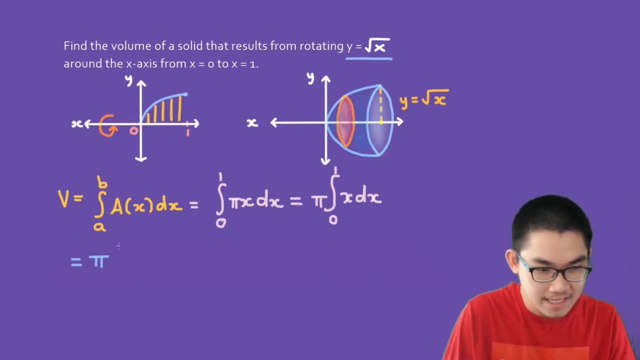 This is the same as pi times the anti-derivative of x which is just 1 over 2 times x to the power of 2. And don't forget the boundaries so up here is 1 down here is 0. 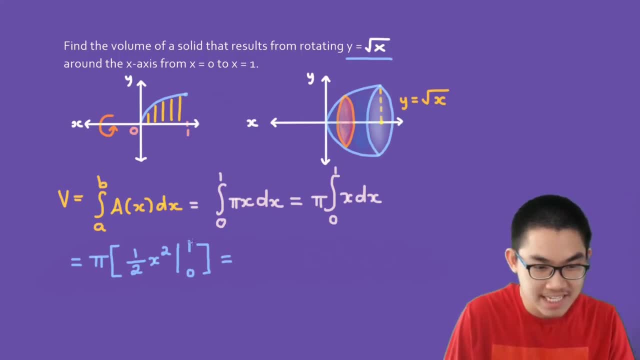 And the final step is just substituting these numbers back into our formula. So this is the same as pi times 1 over 2 times 1 to the power of 2 minus the lower bound which is 0. So 1 over 2 times 0 to the power of 2 and that's it. So we know that this is going to be 1 over 2 and that's going to be 0. So we're going to have pi times 1 over 2. 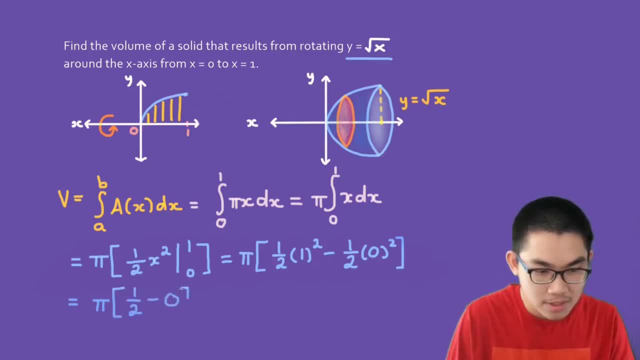 1 over 2 minus 0 which is just pi over 2 and that is our answer. 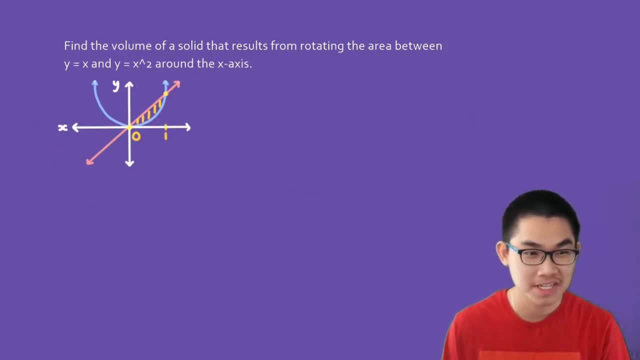 Now let's do one more example of solids of revolution. Find the volume of a solid that results from rotating the area between y is equal to x that's going to be the pink function and y is equal to x square that's going to be the blue function around the x axis. 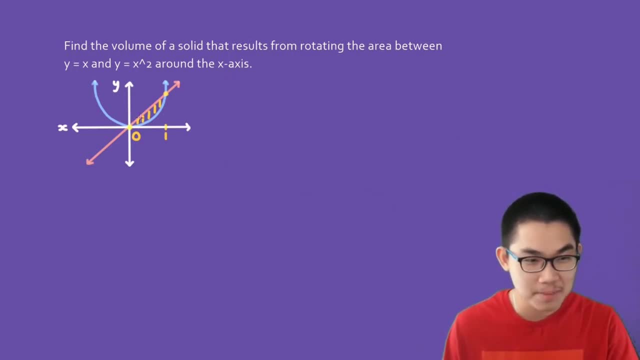 So basically what this is saying is that we have the area between these functions and if we take the function and we rotate it around the x-axis what kind of solid do we have? 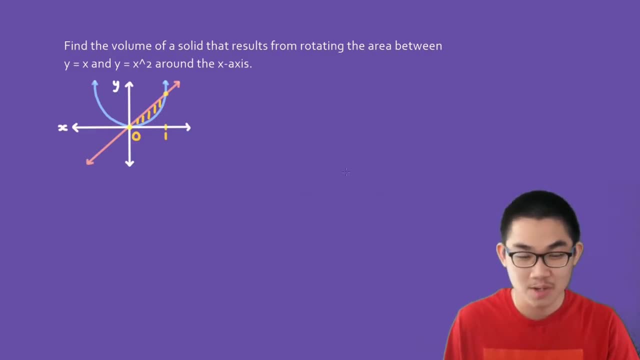 Well it takes a bit of imagination but the solid is going to look like this. 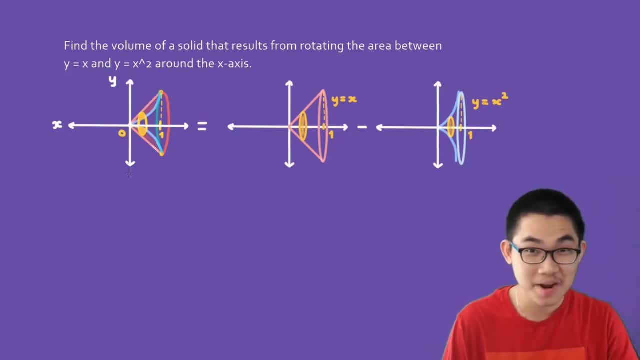 As you can see this solid is a little bit hard to look at so what I did was I break it down into smaller steps. 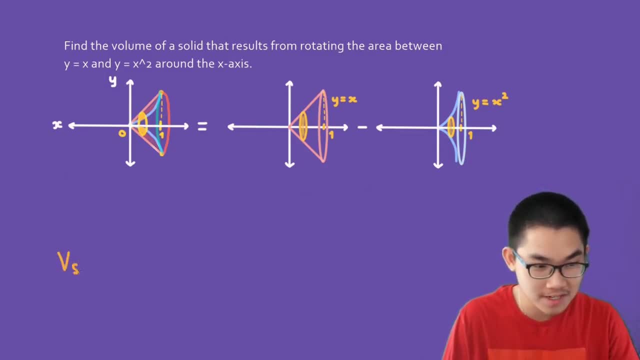 So to obtain the volume of this solid we take the volume of the outside function which is the pink function as you can see so that's the pink function so the volume of the outside function and we minus the volume of the inner function so the volume of the inner function and that will give us the volume of the solid. 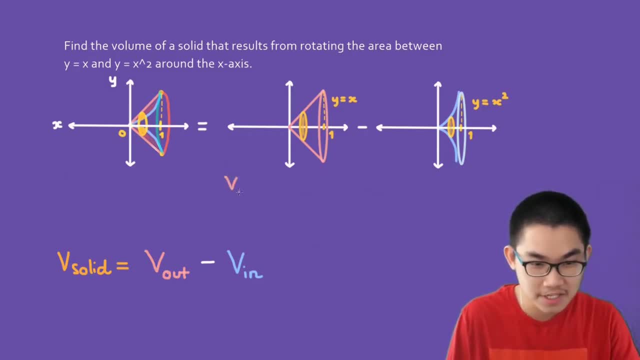 So the volume of this function vout is the same as the integral from 0 to 1 so from 0 to 1 of a of x dx where a of x is the area of the circular cross-section so that's what we need to find first. 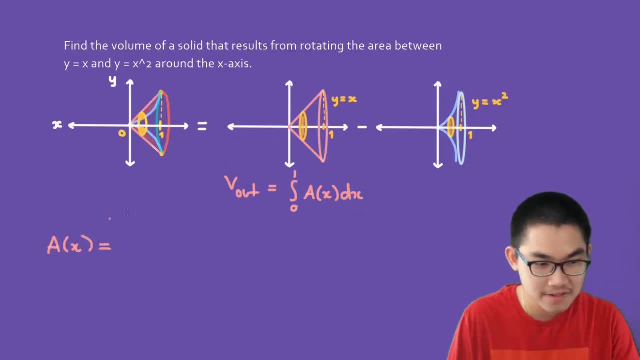 The area of the circular cross-section is the area of the integral from 0 to 1. It's going to be pi times the radius to the power of 2. 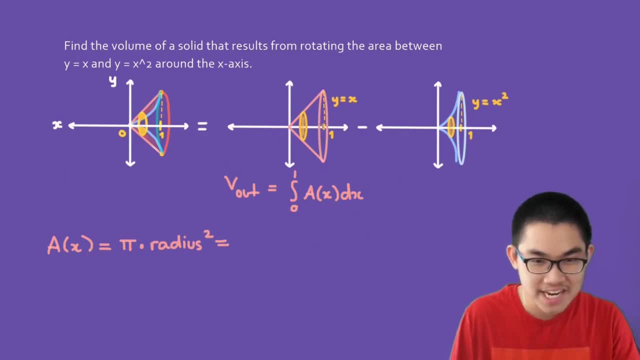 Now if we take a look at this picture we know that the radius is from here to here which is just y and we also know that y is equal to x so we can substitute x into the radius. 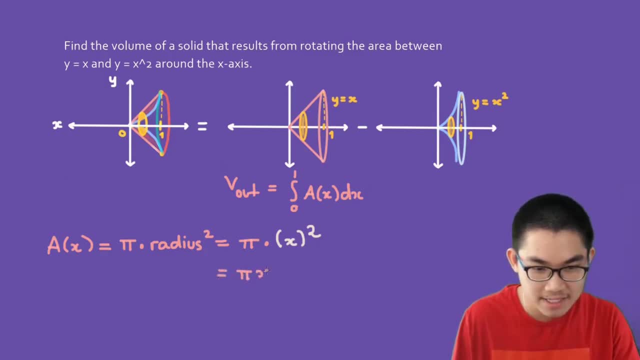 And this is equal to pi times x to the power of 2. 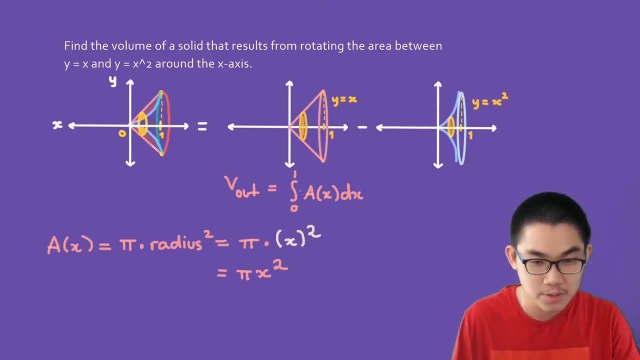 The second step is to substitute this back into this integral so let's go ahead and do that. 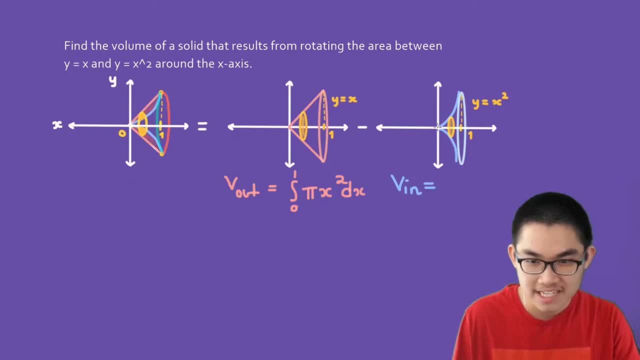 So the volume of the inner function is the same thing the integral from 0 to 1 so 0 to 1 of a of x dx 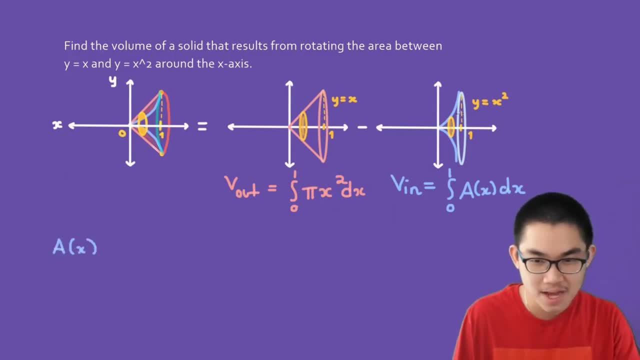 where a of x is the area of this cross-section. So again the area of a circle is pi times the radius to the power of 2 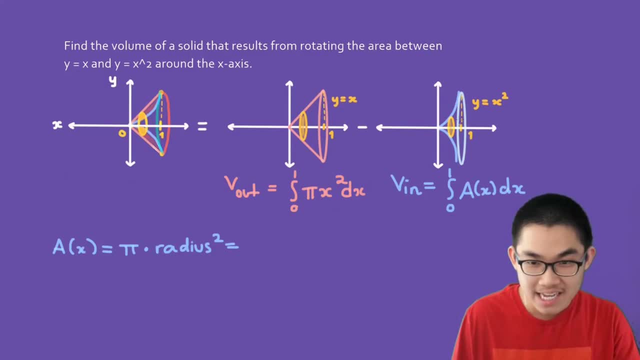 where the radius is y and y is equal to x squared so this is equal to pi times the radius is x squared n to the power of 2. 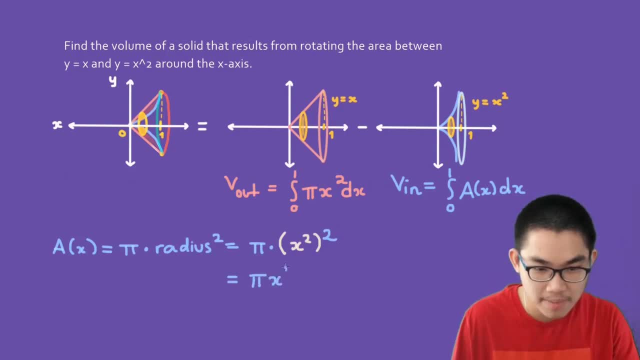 So that will simply be pi x to the power of 4. 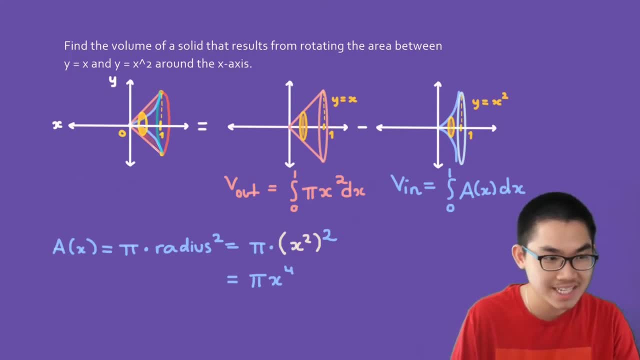 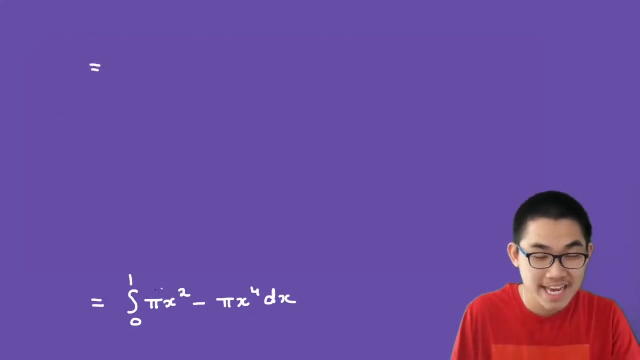 and let's substitute this back into the volume formula so again the volume of this solid the one that we're trying to find is equal to the pink one which is the volume of the outside function so the integral from 0 to 1 i x to the power of 2 dx minus the volume of the inner function so that is the integral from 0 to 1 of pi times x to the power of 4 dx and since both integrals have the same boundaries we can smash them together into one integral and that will simplify a lot of things so this is the same as the integral from 0 to 1 of pi x to the power of 2 minus i x to the power of 4 dx and once again we can take out the pi once again we can substitute out the pi so this is going to be the integral from 0 to 1 of pi times x to the power of 2 minus x to the power of 4 dx and since pi is just a number let's bring it outside of the integral so again i times the integral from 0 to 1 of x to the power of 2 minus x to the power of 4 dx and this is something that we can easily find so this is going to be pi times the anti-derivative of x square which is just 1 over 3 x to the power of 3 and the anti-derivative of x to the power of 4 that's going to be x to the power of 5 and you have to divide by that exponent so divide by 5 and you have to do it from 1 to 0 so don't forget the boundaries guys 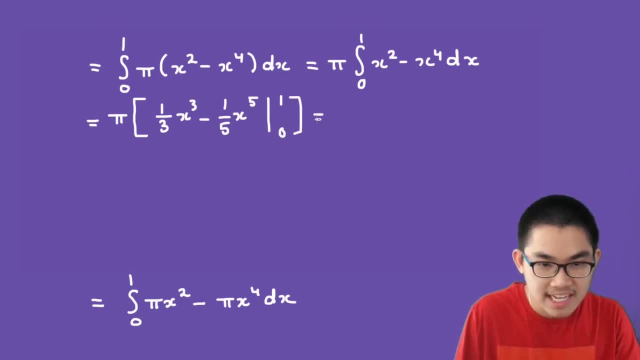 so 1 to 0 now the next step is to substitute these numbers into this formula so let's go ahead and do that let me use yellow this time so pi times this is one over three times one 1 to the power of 3 minus 1 over 5 times 1 to the power of 5 and minus the lower bound which is 0. 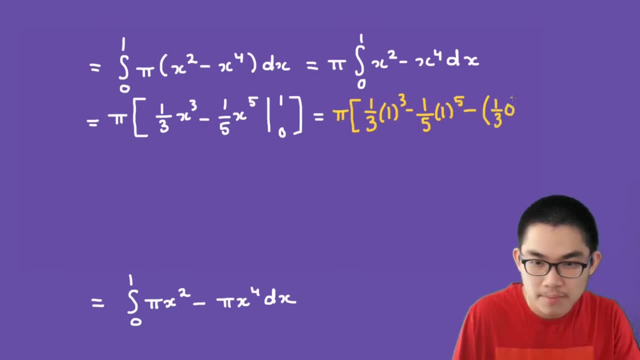 So 1 over 3 times 0 to the power of 3 minus 1 over 5 times 0 to the power of 5 and we can close off the expression right there. So we know that 1 over 3 times 1 to the power of 3 is just 1 over 3. So this is going to be pi times 1 over 3 itself and negative 1 over 5 times 1 to the power of 5 is just negative 1 over 5. And we also know that whatever is here since there's the 0 we know that this whole expression right there is going to be 0. So this is simply minus 0 and all we need to do is solve the fractions. So this is pi times this is going to be 5 over 15 minus 3 over 15 and finally the answer is 2 times pi over 15 so this right here is the 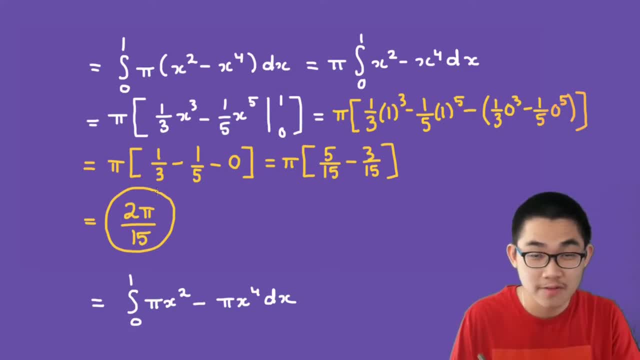 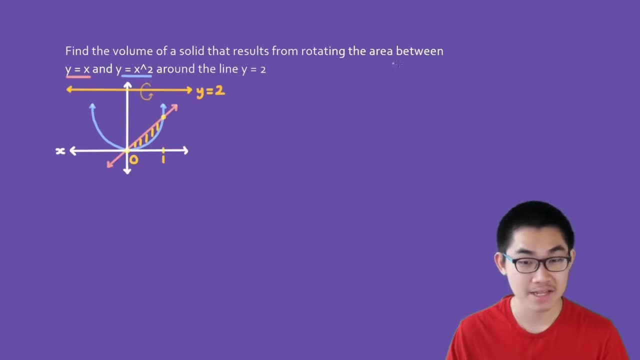 answer and also the volume of the solid of revolution find the volume of a solid that results from rotating the area between y is equal to x that's going to be the pink line and y is going to be equal to x square that's the blue function around the line y is equal to 2 so if you take the area between these two curves and you rotate it around that horizontal line 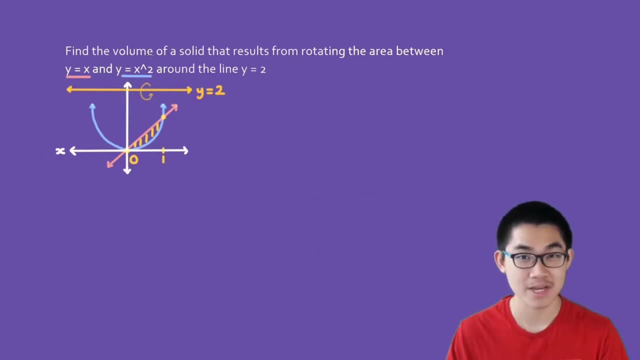 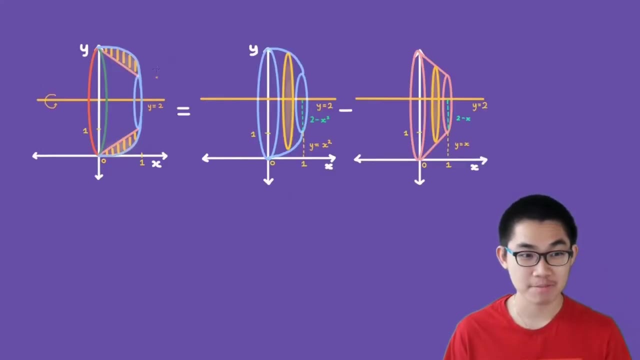 what kind of three-dimensional object are we going to get well we're going to get something like this so as you can see our three-dimensional object is going to look something like this and we want to find the volume of this three-dimensional solid so the volume of this solid is the same as the volume of the outside function so the volume of the outside function minus the volume of the inner function and if you remember from my previous video the formula to find the volume is just the integral from a to b so the integral from a to b and this case it's from 0 to 1. So that's going to be 0, this is going to be 1 of a of x dx. 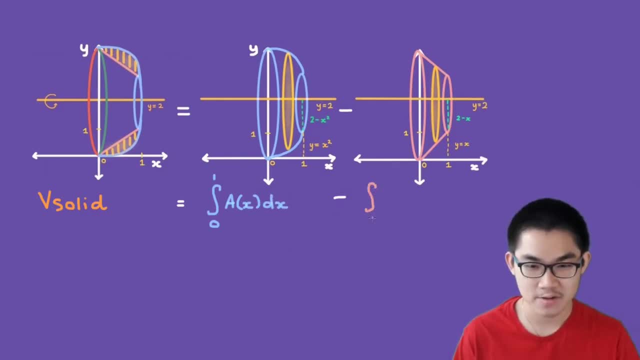 It is the same over here, so that's going to be the integral from 0 to 1 of a of x dx. 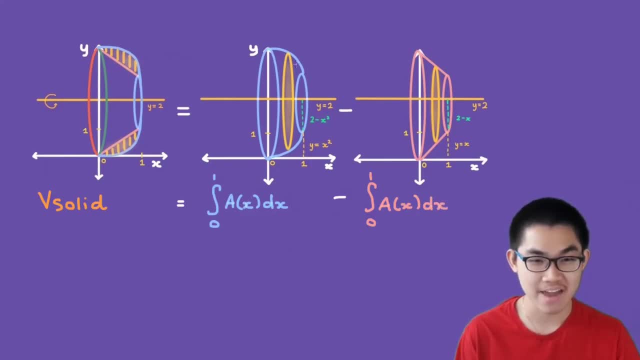 So what is a of x? Well a of x is the area of the cross section which is a circle. So let's write it out. The area of a circle is the same as pi times the radius to the power of 2. And we need to write the radius in terms of x. So this is equal to pi times the radius. And if you look at the diagram, you can see that the radius is from here to here. So how do we find the radius? Well you know that the distance from here to here is 2, that's 2. Because that's y is equal to 2, so the distance is 2. And the distance from here to here is x squared. So the distance in between has to be 2 minus x squared. Pi times 2 minus x to the power of 2, to the power of 2 again. So basically you just take the top y and you minus the bottom y, and that's always going to give you the radius in between. Now the next step is to put this back into our integral. How about the area of the pink cross section? Well again it is just a circle. So the area is just pi times the radius to the power of 2. And we're going to rewrite the radius in terms of x. So this is going to be pi times the distance in between. You take the top y minus the bottom y, that's going to give you 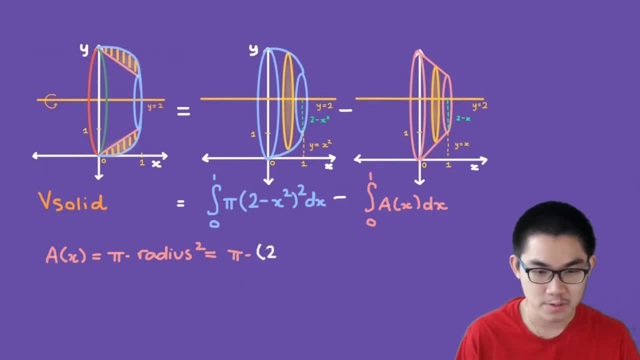 2 minus x. So this is going to be 2 minus x. And don't forget the power of 2 on the top, because that's the radius squared. So let's rewrite this integral in terms of x. 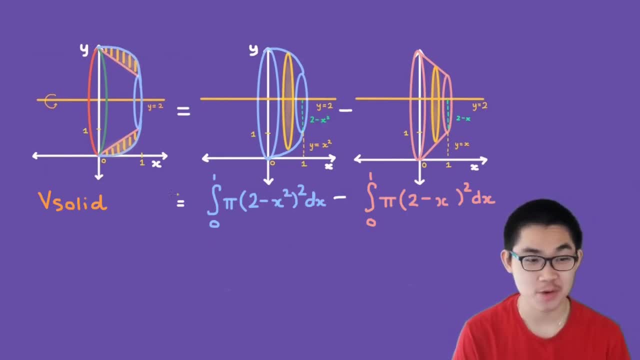 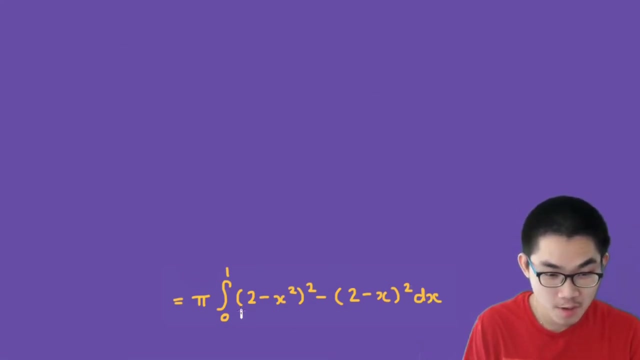 So solving these two integrals will basically give you the volume of this solid. So let's go ahead and do that. And as you can see, since both of them have the same boundaries, we can just match them together into one integral. And that's going to give us the volume of this solid. So let's simplify a lot of things. So this is equal to the integral from 0 to 1 of pi times 2 minus x to the power of 2, to the power of 2, and minus whatever is over there. So minus pi times 2 minus x to the power of 2 dx. And the next step is to factor out the pi. So this is equal to pi times the integral from 0 to 1 of 2 minus x to the power of 2, to the power of 2, and minus 2 minus x to the power of 2 dx. So what we need to do is solve for this right here. So 2 minus x squared to the power of 2 is the same as 2 minus x squared times itself. And don't forget the rules. You have to take this, multiply by this, take this, multiply by that, and the same thing for the other term. So let's go ahead and solve it. 2 times 2 is going to give you 4. 2 times negative x squared is going to give you negative 2x squared. It's the same thing here. So minus 2x squared. And this times that is going to give you positive x to the power of 4. And we can rewrite this as x to the power of 4 minus 4x to the power of 2. 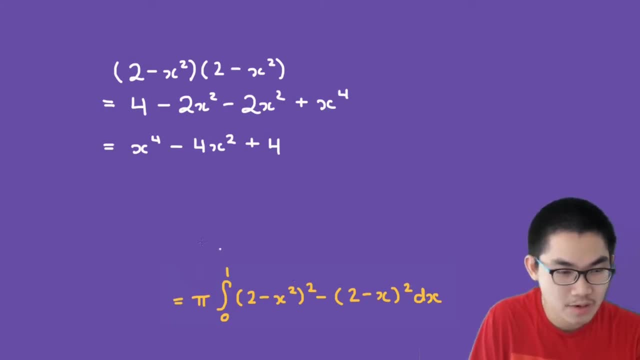 And let's go ahead and put this back into our integral. 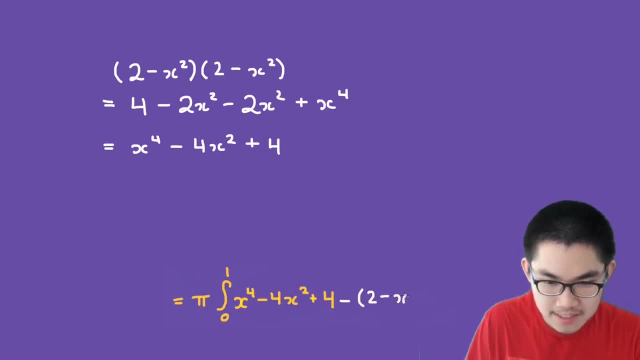 Now minus 2 minus x to the power of 2 dx. So the next step is to solve for this right here. Let's do blue this time. So we have 2 minus x times itself. So 2 minus x. Now 2 times 2 is going to give you 4. 2 times negative x is negative 2x. Negative x times 2 is negative 2x. And negative x times negative x is positive x to the power of 2. And this is the same as x to the power of 2 minus 4x plus 4. So let's put this back into our integral. 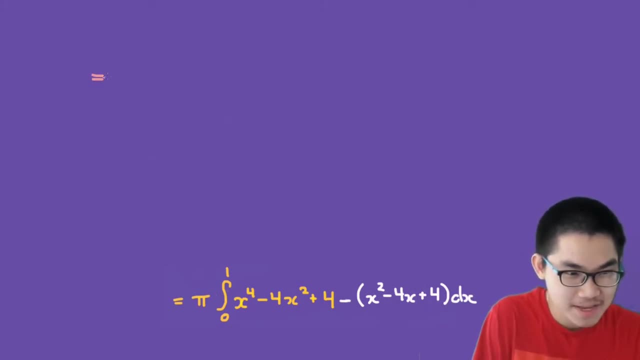 And we are almost done. I'm going to rewrite this. This is going to be pi times the integral from 0 to 1. We have x to the power of 4 minus 4x. And we are almost done. So let's go ahead and solve for this right here. So this is 4x to the power of 2 plus 4 and minus negative x to the power of 2 plus 4x and minus 4dx. 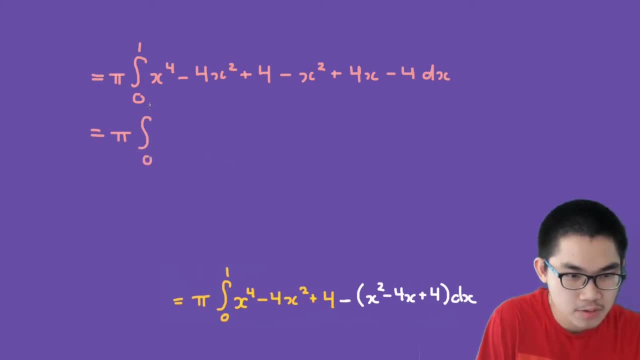 So this is again equal to pi times 0 to 1 x to the power of 4. And negative 4x squared minus x squared is going to give you negative 5x squared. And 4 minus 4x to the power of 2 minus 4dx. And 4 minus 4 is just 0. So the last thing we have is just this one. So plus 4xdx. And time to integrate this integral. This is going to be the same as pi times the antiderivative of x to the power of 4, which is just 1 over 5 x to the power of 5. The antiderivative of negative 5x squared is negative 5 over 3 x to the power of 3. And lastly, the antiderivative of 4x is negative 5 over 3 x to the power of 3. So this is just 4 times x to the power of 2 over 2, which is just 2 times x squared. And the boundary goes from 1 to 0. So again, this is the same as pi times 1 over 5 minus 5 over 3 plus 2. So that's after plugging in these variables. And it's just a matter of solving these fractions now. 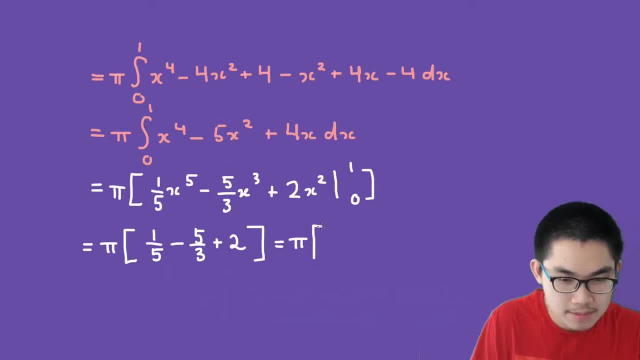 So this is the same as pi. So this is pi times 3 over 15 minus, this is going to be 15, that's going to be 25, plus 30 over 15. 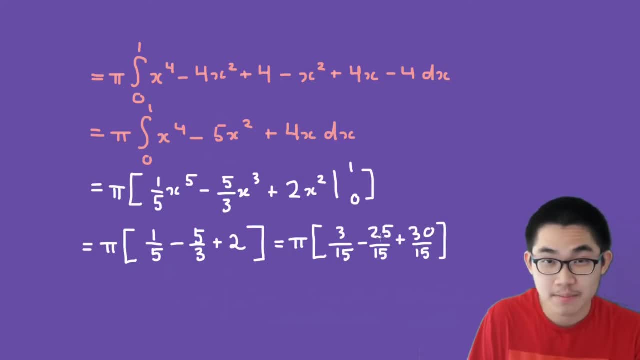 So 30 minus 25 is positive 5. And positive 5 plus 3 is 8. So the final answer should be pi times 8 over 15. 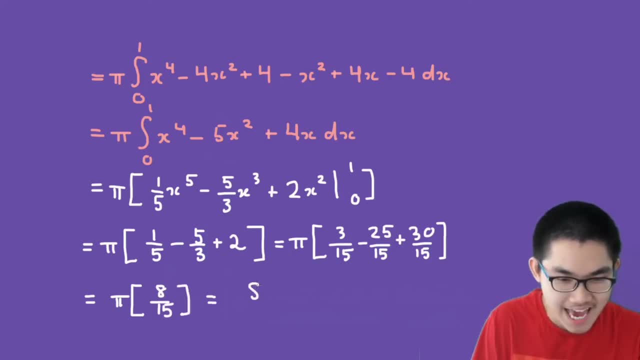 And one final step. This is just a simple equation. So this is the same as 8 times pi over 15. 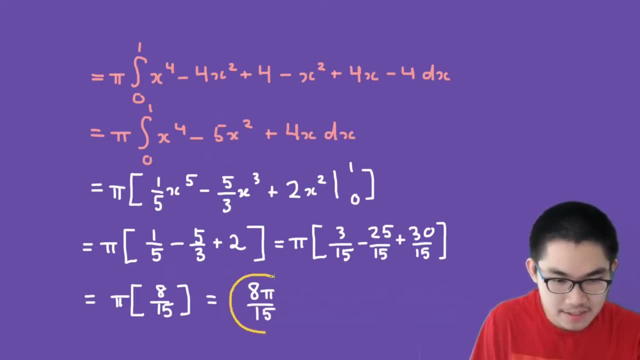 And this right here, so this right here is the volume of our solid of revolution. So let's take a look at this problem. 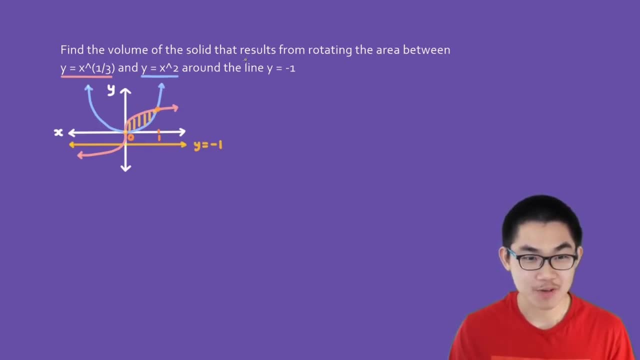 Find the volume of the solid that results from rotating the area between y is equal to x to the power of 1 third. That's going to be the pink function. 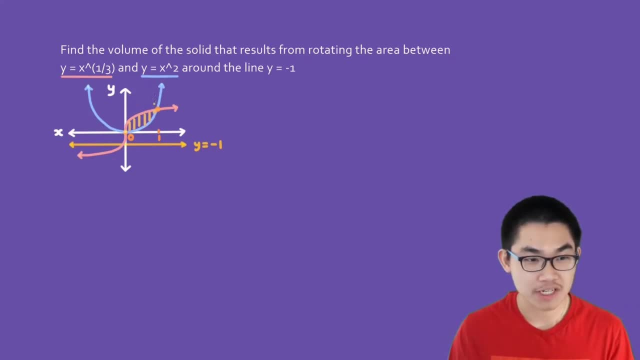 And y is equal to x squared. That's the blue function around the line y is equal to negative 1, which is the yellow line. 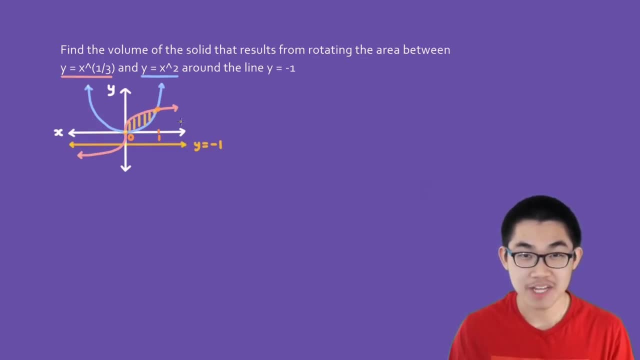 So imagine you take the area between these two curves and you rotate it around the yellow line. Well, what kind of object are you going to get? 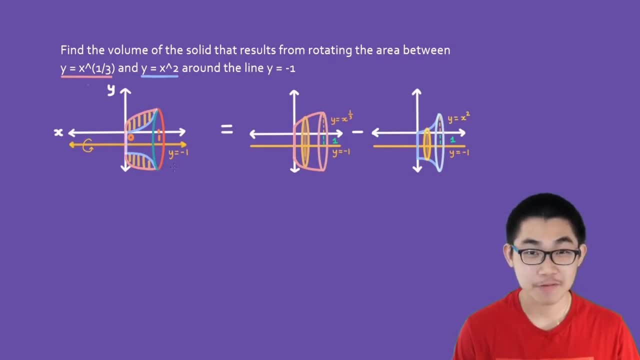 So you're going to get something like this. And to find the volume of this three-dimensional solid, all you have to do is take the volume of the outside function, which is the pink function, that's the outside function. 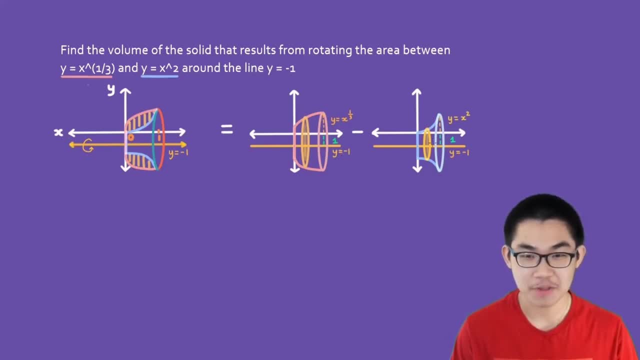 And you minus the volume of the inner function, which is the blue function. So let me repeat that. 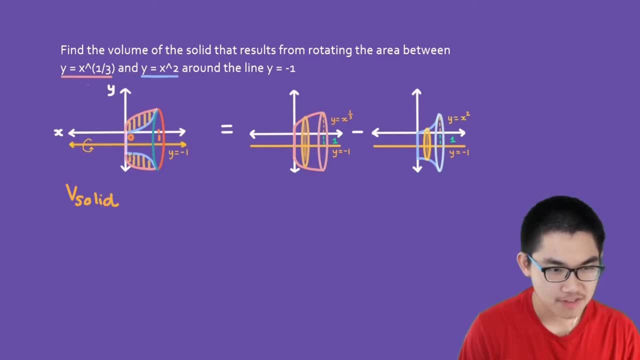 The solid, which is the volume of this solid, is equal to the volume of the outside function minus the volume of the inner function. 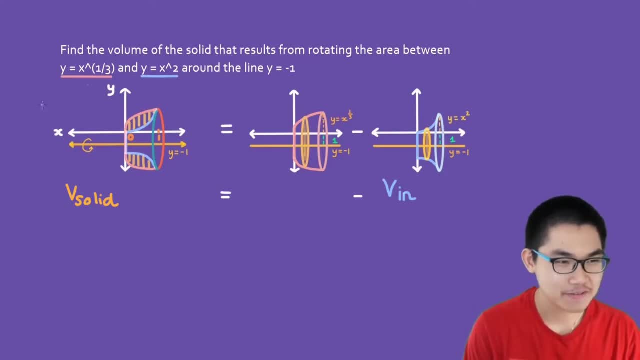 So what is the formula for the volume? 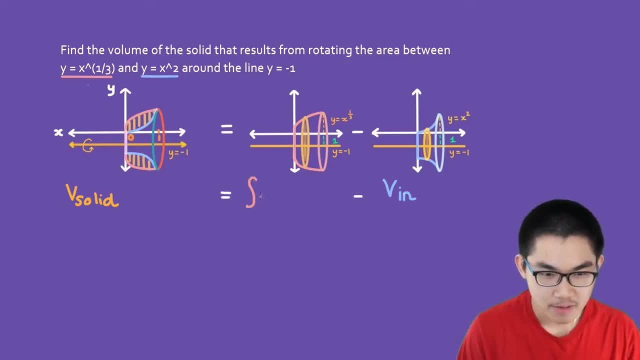 volume of solids well it's basically the integral from a to b but in this case we just want to find the volume from 0 to 1. so that's going to be 0 to 1 of a of x dx where a of x is the area of the circular cross section for the volume of the inner function it is the same thing so zero to one of a of x dx so a of x is a circle so that's going to be pi times the radius to the power of 2 which is equal to pi times now if you take a look at the diagram you know that the radius is the distance from this line to the top right and so you know that the distance from here to here is x to the power of 1 so that's going to be pi times the radius to the power of 2 which is equal to pi times third and the distance from here to here is going to be one and so the radius will simply be x to the power of one third plus one now there is one formula that will always give you the radius let me show you what it is so the radius can also be found using this formula 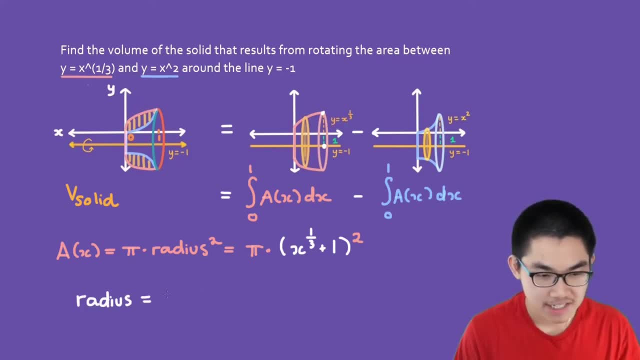 you take the top y which is x to the power of one third and you minus the bottom y 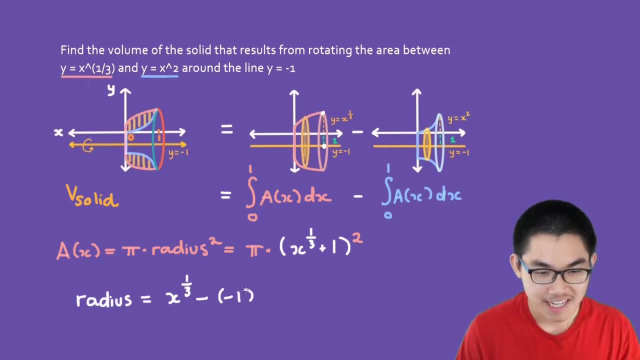 which is negative one so that's going to give you x to the power of one third plus one which is the same as the one we found so you can either find the radius by looking at the diagram or just use 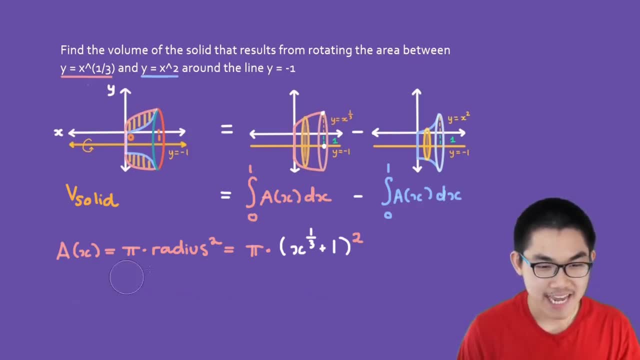 this formula so the next step is just putting this back into our integral right there the area of the blue circular cross section is the same it's just pi times the radius squared 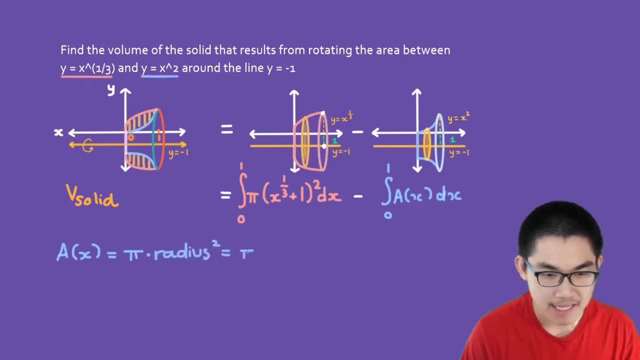 because it's a circle so that's equal to pi times now the radius is from here to here so we take this distance well that's going to be x to the power of 2 plus this distance right there 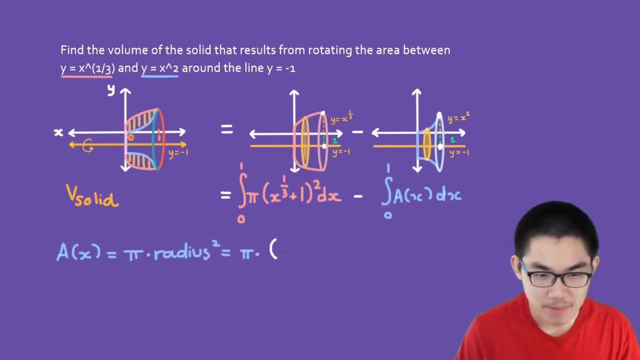 which is just 1, to the power of 2. So the other way to find the radius, if you prefer the second 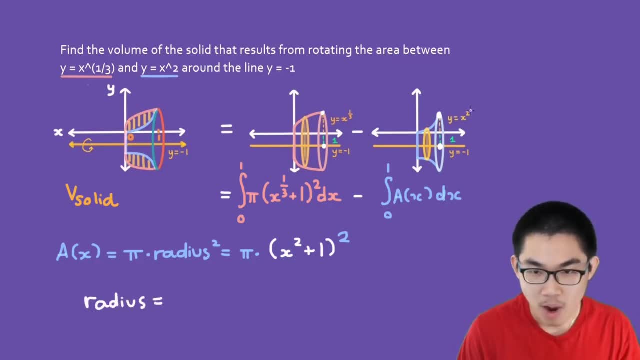 way, is just to take the top y, so take the top y, and we know that y is the same as x to the power of 2, and you minus the bottom y, so minus negative 1, but that's also going to give you x squared plus 1, which is the same as the radius we just found. So you can use either way, whichever 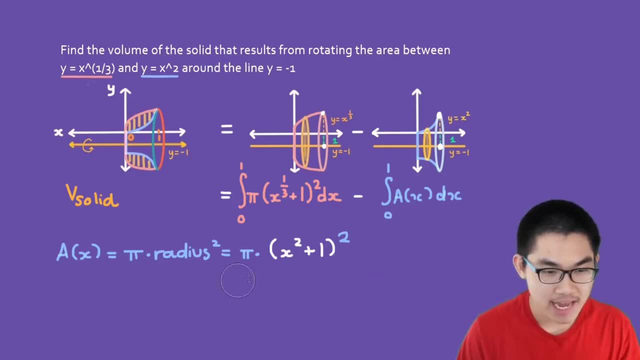 you prefer. And let's go ahead and put this back into our integral. 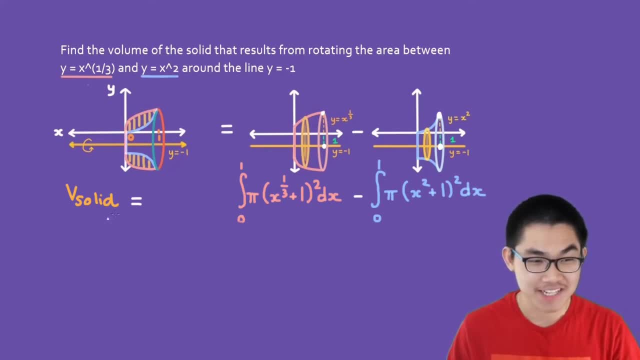 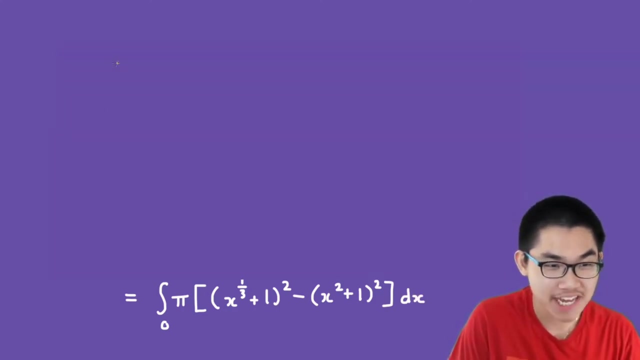 We are ready to find the volume of this solid. So since both integrals have the same boundaries, we can just match them together into one integral, and that's going to simplify the problem. So let's go ahead and put this back into our integral. So this is the same as the integral from 0 to 1 of pi times x to the power of 1 third plus 1 to the power of 2 minus pi times x to the power of 2 plus 1 to the power of 2 dx. So the next step is we can just factor out the pi. That's going to be the same as the integral from 0 to 1 times pi times x to the power of 1 third plus 1 to the power of 2 minus x to the power of 2 plus 1 to the power of 2 dx. Since pi is just a number, we can bring it outside of the integral. So that's going to be the same as pi times the integral from 0 to 1 times x to the power of 1 third plus 1 to the power of 2 minus x to the power of 2 plus 1 to the power of 2 dx. Now what we need to do is we need to solve this right here. So first of all, what is x to the power of 1 third plus 1 to the power of 2? Well, that's just the same as x to the power of 1 third times itself. So remember, you have to use a formula. You've got to multiply this by x to the power of 1 third plus 1 to the power of 2. 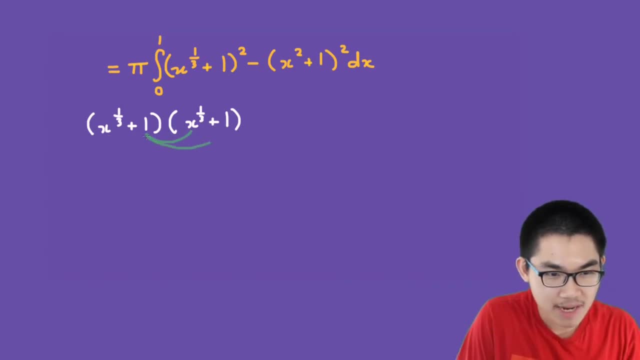 Multiply that plus this multiplied by that. That's going to be the same as x to the power of 1 third to the power of 2 because we multiply these together plus x to the power of 1 third times 1. That's x to the power of 1 third plus 1 times x to the power of 1 third. And finally, plus 1. 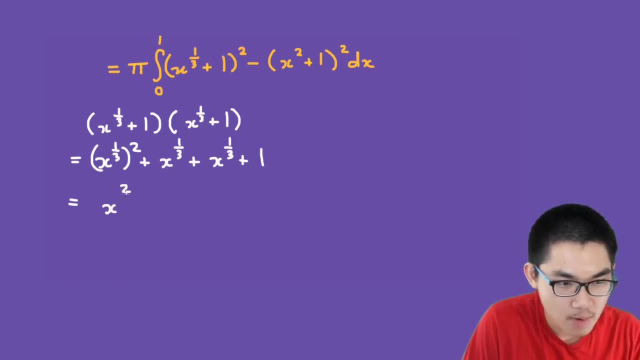 So this is going to be the same as x to the power of 1 third times 1 to the power of 2. of 2 thirds plus 2 times X to the power of 1 third plus 1. So let's go ahead and rewrite this. 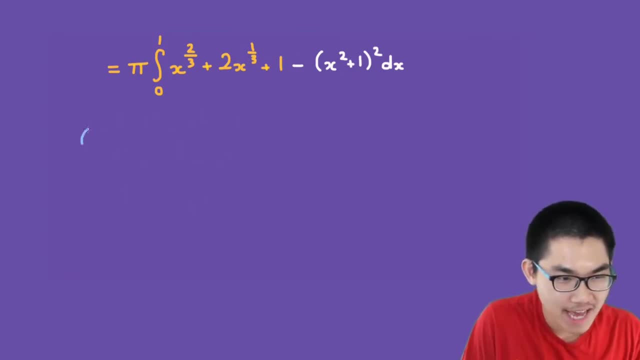 For this one right here that's gonna be X to the power of 2 plus 1 times X to the power of 2 plus 1 again and so X to the power of 2 times X to the power of 2 that's gonna be X to the power of 4 plus X to the power of 2 times 1 that's X to the power of 2 so 1 times X to the power of 2 is X to the power of 2 and 1 times 1 is just 1. So again this is the same as X to the power of 4 plus 2 X to the power of 2 plus 1. So let's put it back into here. You 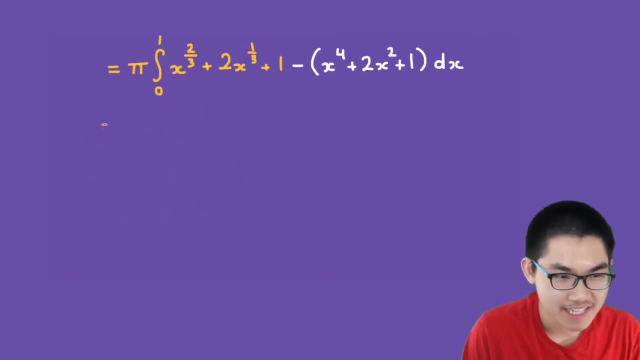 so let's rewrite this. This is gonna be the same as pi times the integral from 0 to 1 of X to the power of 2 thirds plus 2 times X to the power of 1 third plus 1 minus X to the power of 4 minus 2 times X to the power of 2 and minus 1 DX. Of course the one 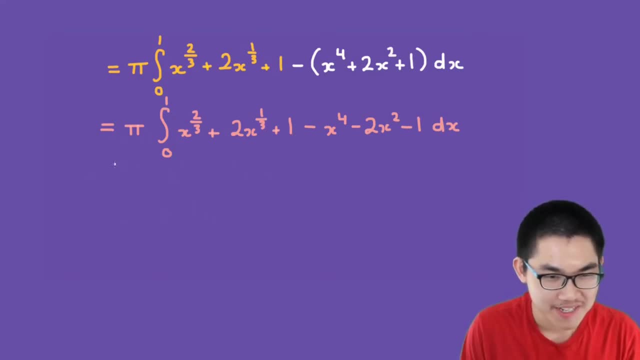 are going to cancel out because 1 minus 1 is 0 so this is going to be pi times the integral from 0 to 1 of x to the power of 2 thirds plus x to the power of 1 third minus x to the power of 4 minus 2 times x to the power of 2 dx and so let's integrate it this is going to be pi times the integral or sorry the anti-derivative of x to the power of 2 thirds this is going to be x to the power of 5 thirds and you have to divide by this exponent so divide by 5 over 3 well that's the same as 3 over 5 right there the anti-derivative of 2 times x to the power of 1 third so let's do that this is going to be 4 over 3 and you have to divide by 5 over 3 and you have to divide by 5 over 3 divide by the exponent so divide by 4 over 3 well that's the same as 2 times 3 over 4 times x to the power of 4 over 3. so this right there that's going to simplify into 3 over 2 so let's rewrite that 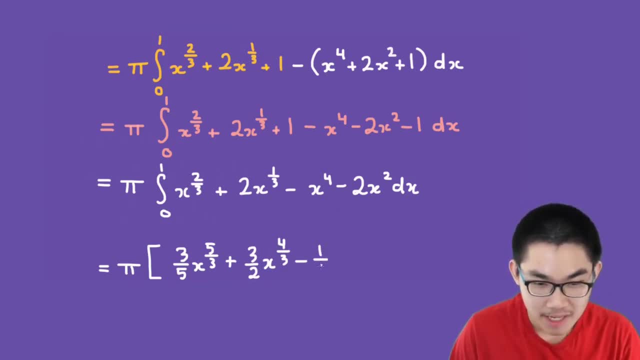 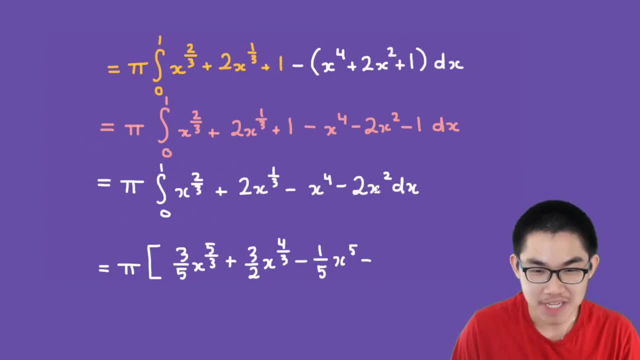 finally the anti-derivative of negative 2 times x to the power of 2 is 2 over 3 times x to the power of 3 and the boundary goes from 1 to 0 so that's going to be 1 this is going to be 0 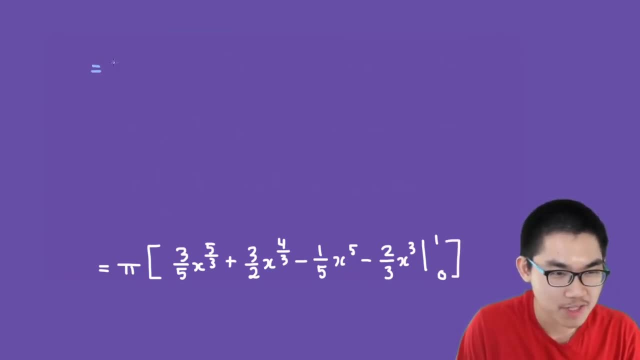 it's time to solve for this it's just a matter of solving so pi times 3 to the power of 5 times 1 to the power of 5 over 3 so we're basically substituting the top number the upper limit so this is plus 3 over 2 times 1 to the power of 4 over 3 minus 1 over 5 times 1 to the power of 5 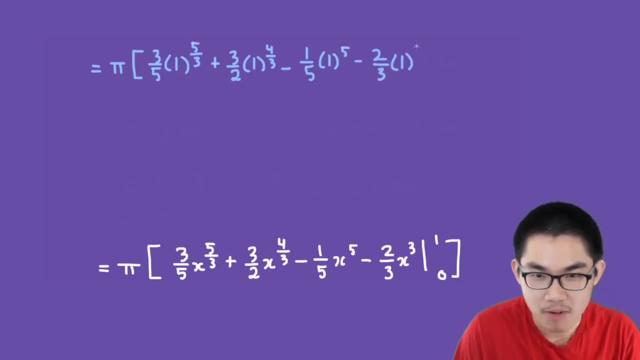 minus 2 over 3 times 1 to the power of 3 and time 2 minus the lower bound so that's what we have to do so we're just going to minus the lower bound the lower bound is just going to be 3 over 5 times 0 to the power of 3 over 5 plus 3 over 2 times 0 to the power of 4 over 3 minus 1 over 5 times 0 to the power of 5 and minus 2 over 3 times 0 to the power of 3. well but if you look 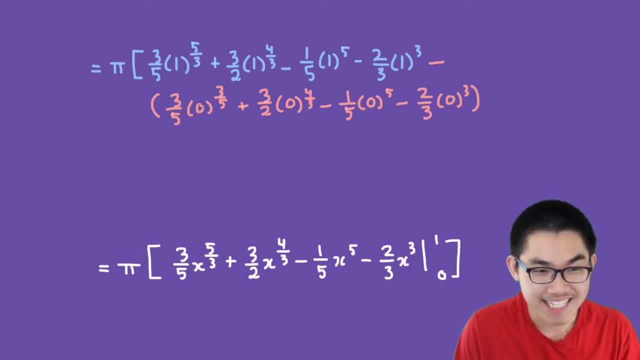 at this you know that's going to be 0 right away because that's going to be 0 and 0 times any number is 0 so the same for all of this so this right there that's going to be zero 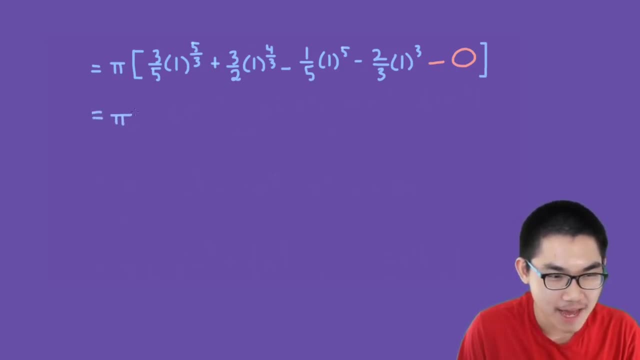 we are so close to finishing so again this is just pi times this is going to be 1 times 3 over 5 which is just 3 over 5 plus this is going to be 3 over 2 this is going to be negative 1 over 5 minus 2 over 3 so it's just a matter of matter of solving fractions the common denominator is going to be 30 so pi times this is 30 that's going to be 18 plus this is going to be 30 and that's going to be 45 minus that's going to be 30 this is going to be 6 and minus 20 over 30 and finally 18 plus 45 minus 6 minus 20 is just going to give you 37 so this is pi times 37 over 30 and the final answer is just going to be 37 over 30 times pi so this right there so this right here represents 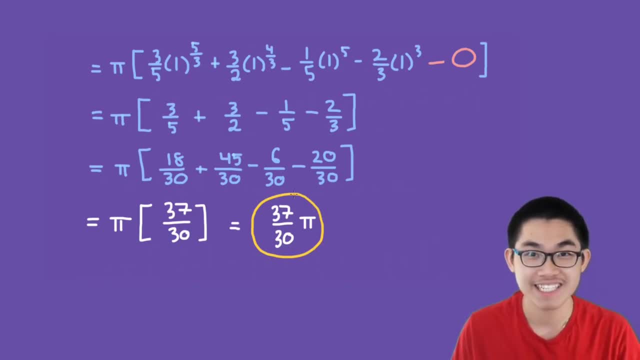 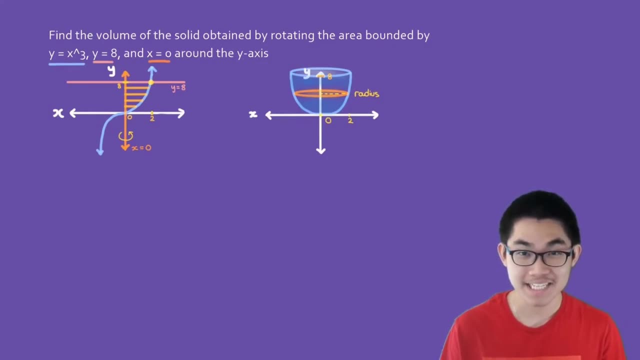 the volume of our three-dimensional solid in this video we're going to talk about solids of revolution but instead of rotating around the x-axis we're going to rotate around the y-axis. So let's take a look at an example. Find the volume of the solid obtained by rotating the area bounded by y is equal to x to the power of 3, that's gonna be the blue function right here, and y is equal to 8, which is the pink function, and x is equal to 0, and we rotate the area around the y-axis. And so if we take the area between these curves, and we rotate it around the y-axis, what kind of three-dimensional 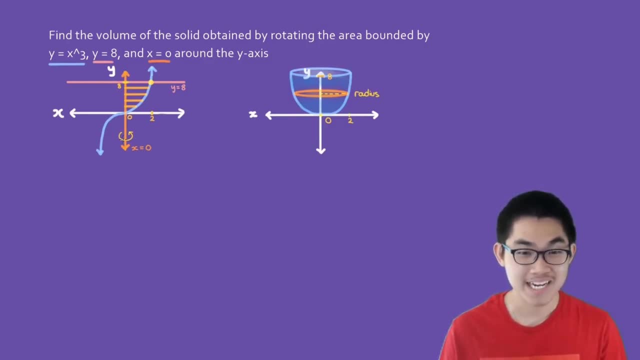 object are we gonna get? Well, we're gonna get something like this, and this is the solid that we want to find the volume of. So to find the volume, we need to write down the volume formula, which is v is equal to the integral from a to b of a of y dy. 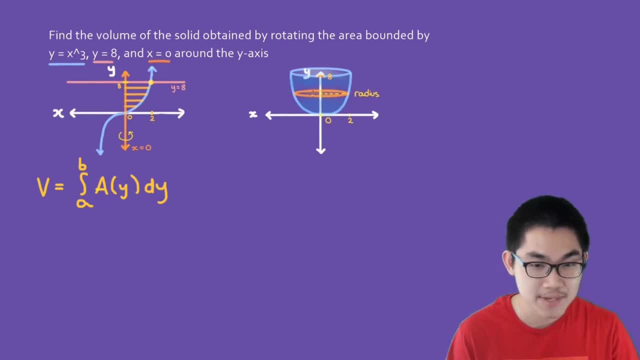 And the reason that we are integrating with respect to y is because the cross section, which is a circle, is sitting on the y-axis, which makes it easier to integrate with respect to y. And the limit from a to b is simply from 0 to 8, so we can fix that. So the limit is just from 0 to 8. 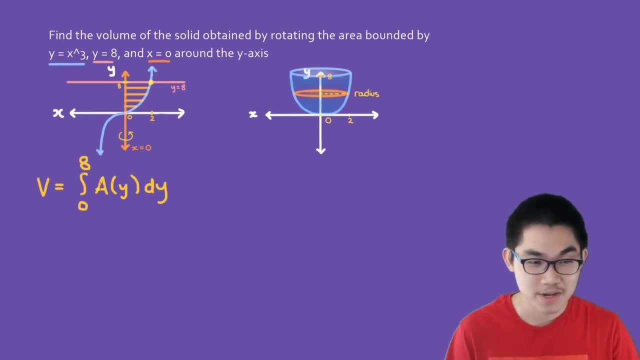 The next step is to find the area, and so we know that the area is the cross section, 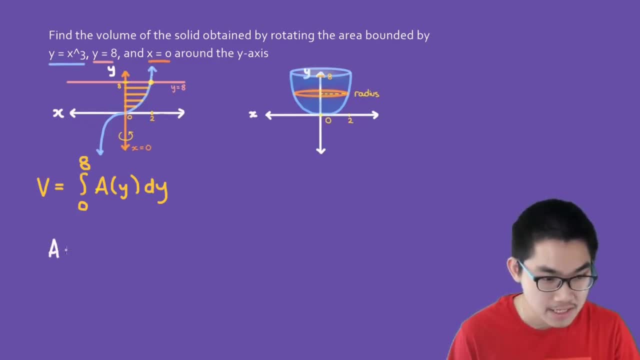 a circle and the area of a circle is the same as pi times the radius to the power of two and how do we find the radius well let me show you how to do that so first of all we know that the distance from the center to the cross section is y we can simply call that y and we also know that the distance from the y-axis so from here until it touches the function which is there is x so we know that's x which means that the radius has to be equal to x so let me rewrite this this is the same as pi times the radius which is just x to the power of two so to the power of two and we need to rewrite this in terms 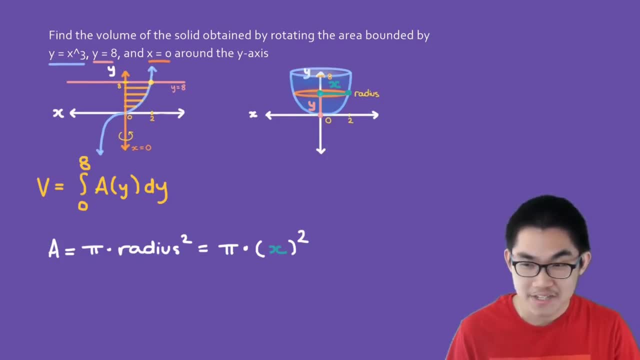 of y because we're integrating with respect to y and so we know that this function is the same as y is equal to x to the power of three which means x is the same as y to the power of one third so this is the same as pi times y to the power of one third to the power of two which is simply pi times y to the power of two thirds so we successfully found the area formula and it's time to put it back into our integral 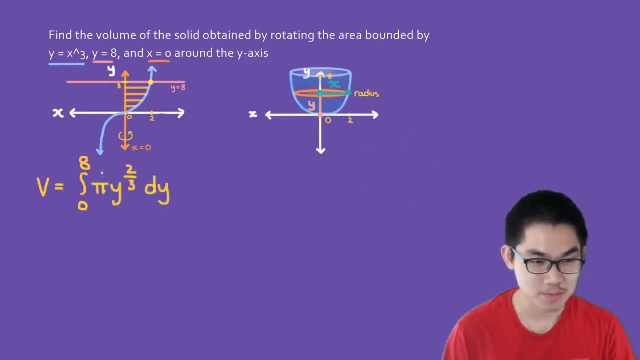 the last step is to evaluate this integral which will basically give you the volume of this solid so the first thing that we notice is that pi is a constant so we can just bring it outside of the integral so this is equal to pi times the integral from 0 to eight of y to the power of two-thirds dy which is the same as pi the antiderivative of y to the power of two-thirds so first of all this is going to be y to the power of five-thirds and then you have to divide by the exponent which will basically give you three over 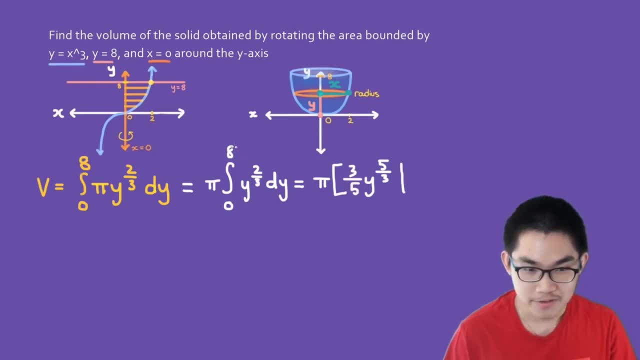 five right here and don't forget the boundaries you have to do it from zero to eight so the top one will be eight the bottom will be zero so the next step is to substitute in these limits and if you do that we're going to get pi times three over five times eight to the power of five over three minus three over five times zero to the power of five over three this is going to be the same as pi times three over five times thirty-two so if you evaluate eight to the power of five of 5 over 3 you're gonna get 32 and this will simply be 0 so minus 0 right here and finally this is PI times 96 over 5 and the answer will simply be 96 divided 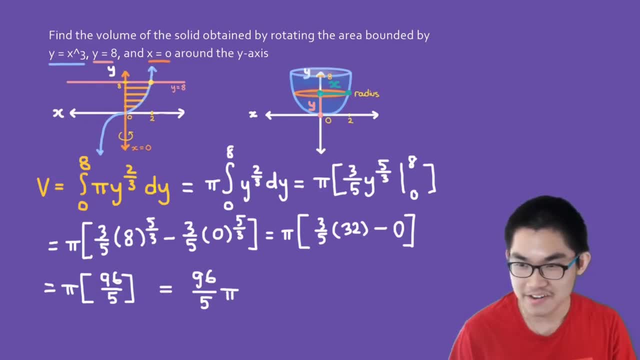 by 5 PI so this right here this number right here 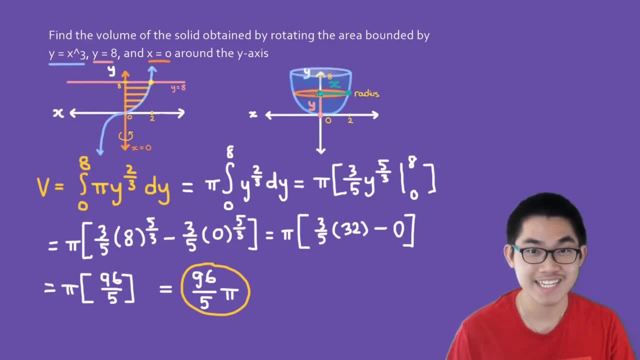 represents the volume of this solid so let's go ahead and do the next problem 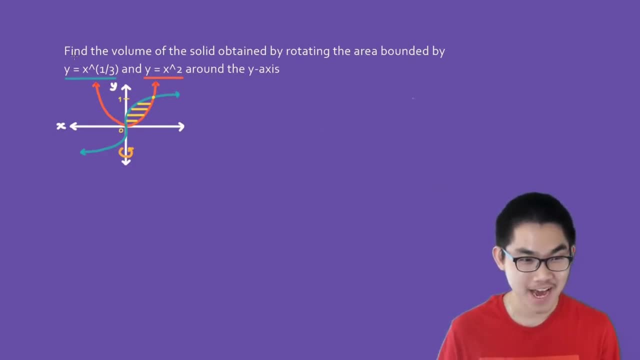 okay next problem find the volume of the solid obtained by rotating the area between y is equal to x to the power of one-third that's going to be the green curve right here and y is equal to x squared which is the red function around the y-axis so imagine if you take the area between these two curves and then you rotate it around the y-axis what kind of 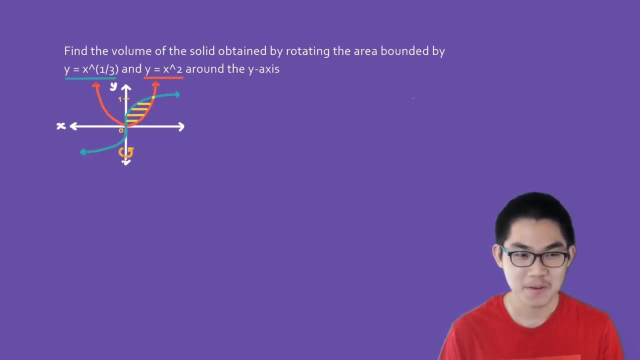 three-dimensional object are we gonna get well we're gonna get something like this as you can see our solid is gonna look like this and the volume of this solid is the same as the volume of the outside function and the outside function is y is equal to x square minus the volume of the inner function so y is equal to x to the power of one-third so let me repeat that the volume of our solid is the same as the volume of the outside function minus the volume of the inner function so we know that the volume formula is just the integral from a to b and in this case it's going to be 0 to 1 so this is 0 this is 1 of a of y dy where a of y is the area of the circular cross-section. How about the volume of the inner function? Well, it's going to be the integral from a to b, it's 0 to 1, of a of y dy. 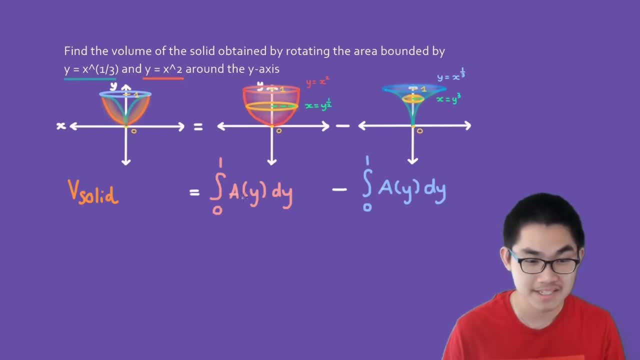 The next step is to find the area formula. So for this area, we know that the area is going to be pi times the radius to the power of 2, because that's the area formula for a circle. And so we also know that the distance from the center to the cross-section is y, we can call that y. And so the distance from the y-axis until it reaches the outer edge of the function, which is here, so this distance right here is x. And since y is the same as x to the power of 2, we solve it, we solve for x, and we're going to get x is equal to y to the power of 1 half. And so the radius, let me rewrite this, this is equal to pi times x to the power of 2. And x is simply y to the power of 1 half. So this is the same as pi times y to the power of 1 half to the power of 2, which is equal to pi. 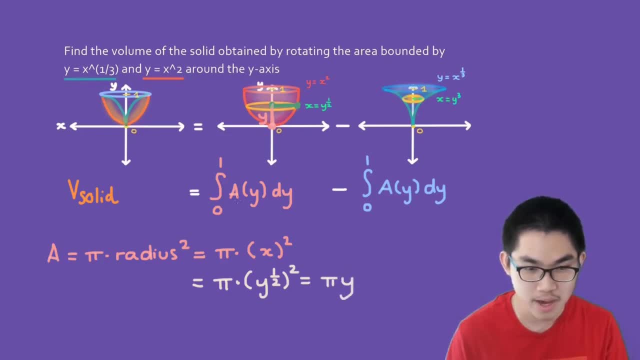 times y. Now let's put this back into our integral. 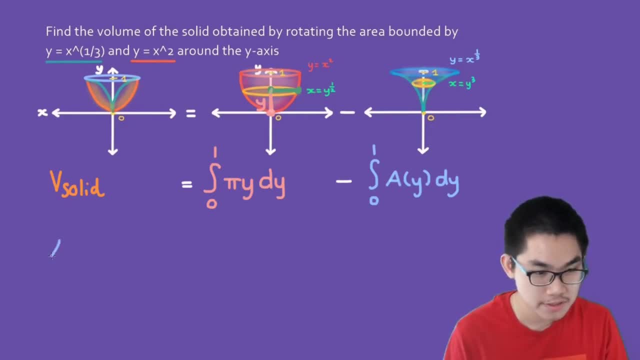 Now the area of the blue circular section is also a circle, so that's going to be the same as pi times the radius to the power of 2. And again, we know that the distance from the center to the cross-section, so this distance right here, is going to be y. So that distance, this is y, and the distance between the y-axis until it reaches the edge of the function, so this distance is going to be x. So if we solve this, we're going to get x is equal to y to the power of 3. So let's rewrite this function, we're going to get pi times x to the power of 2. And since x is just y to the power of 3, we're going to get pi times x to the power of 2. And this is simply equal to pi times y to the power of 6. So let's go ahead and put this back into our integral right here. 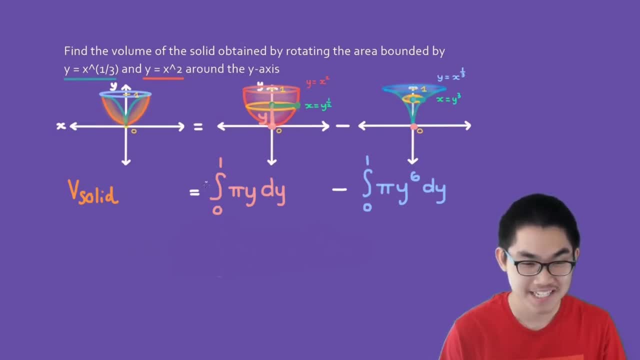 We are so close to finishing. So since both of these integrals have the same boundaries, we can just smash them together into one integral, and that's going to simplify a lot of things. 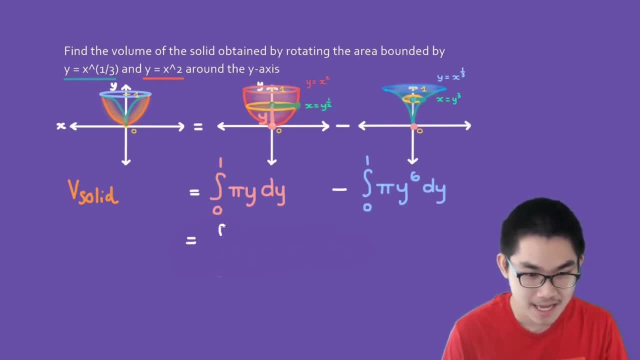 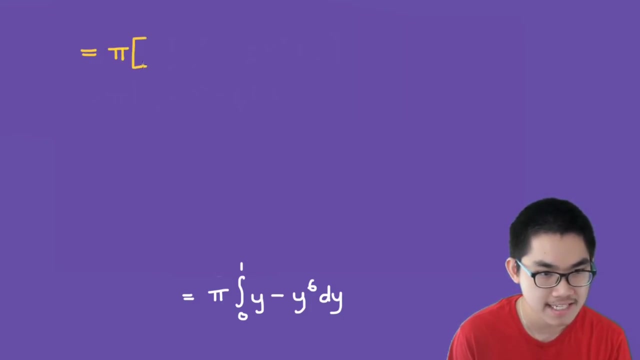 So the volume of the solid is the same as the integral from 0 to 1 of pi times y minus this pi times y to the power of 6 dy. And again, since pi is just a number, we can bring it outside of the integral. So this is equal to pi times the integral from 0 to 1 of y minus y to the power of 6 dy. This right here is the same as pi times the antiderivative of y, which is just 1 over 2 times y to the power of 2 minus the antiderivative of y to the power of 6. That's just 1 over 7 times y to the power of 7. And don't forget the boundaries, that goes from 0 to 1. Now this is the same as pi times 1 over 2. 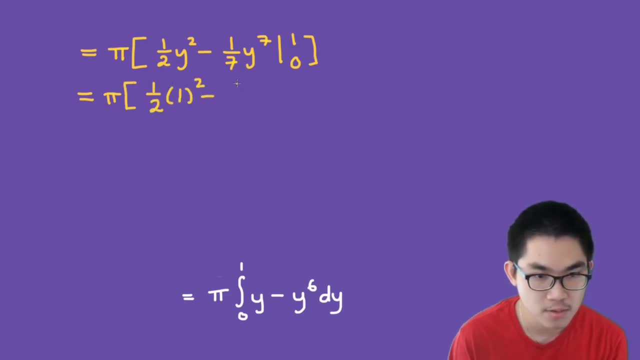 So this is equal to pi times 1 to the power of 2 minus 1 over 7 times 1 to the power of 7 and minus the lower bound. So the lower bound will simply be 1 over 2 times 0 to the power of 2 minus 1 over 7 times 0 to the power of 7. And we're going to go ahead and close off the bracket right here. 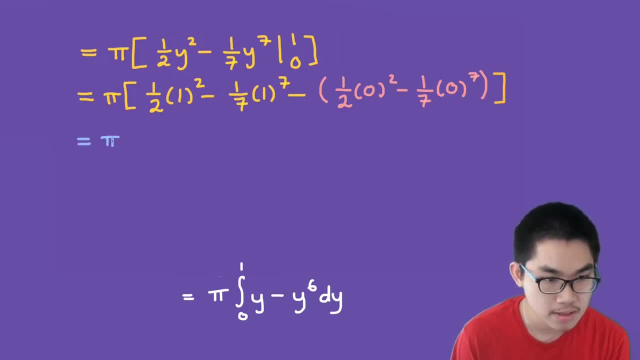 So the next step is simplifying the whole thing. So pi times 1 over 2 minus 1 over 7. And we know that this whole thing right here, that whole expression is just going to be 0. So this is equal to pi times 7 over 14 minus 2 over 14. And the answer 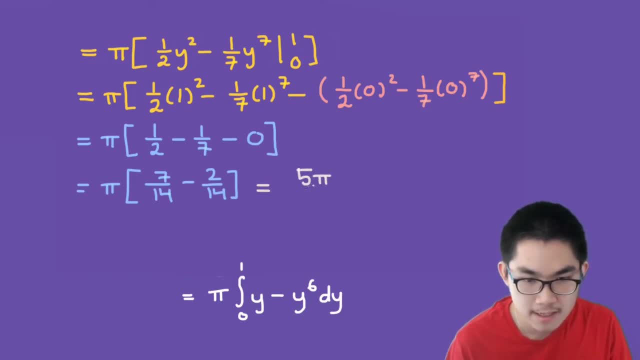 will simply be 5 times pi over 14. So this number right here, so let me circle it, this number right here represents the volume of our solid. In this video we're gonna find the volume 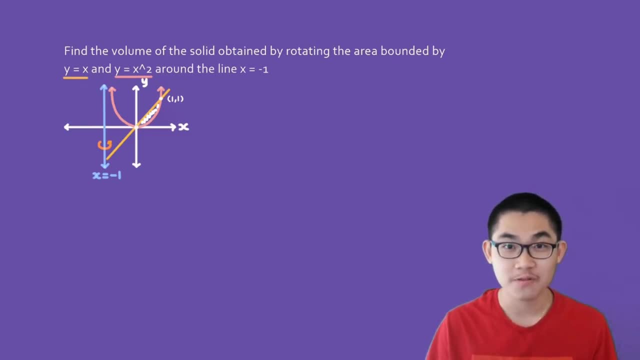 of solids of revolution rotated around vertical lines to the left of the y-axis. So let's take a look at this problem, find the volume of the solid obtained by rotating the area bounded by y is equal to x, that's going to be the yellow line. And y is equal to x to the power of 2. And so if we take it, take the area between these two curves and we rotate it around x is equal to negative one so this vertical line and if we rotate it around this line what kind of three-dimensional solid are we going to get well we're going to get something like this so our three-dimensional object is going to look something like this and we want to find the volume of this object 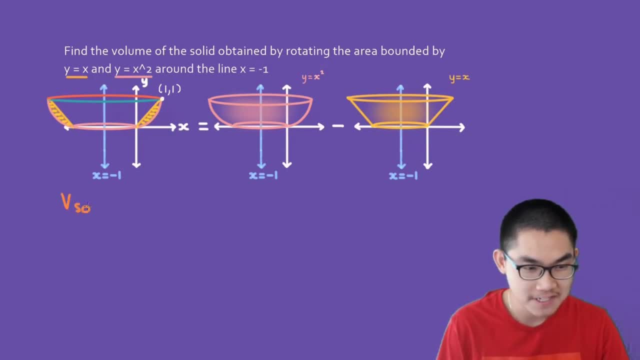 so the volume of this solid or v solid is equal to the volume of the outside function so v out minus the volume of the inner function so v in now if you look at the diagram when we rotate the area around the curve we're going to have some empty space inside and so to get rid of that empty space we need to find the volume of the outside function side function which is y is equal to x to the power of 2 and we minus the volume of the inner function and that's basically going to get rid of all of the empty space inside all right so 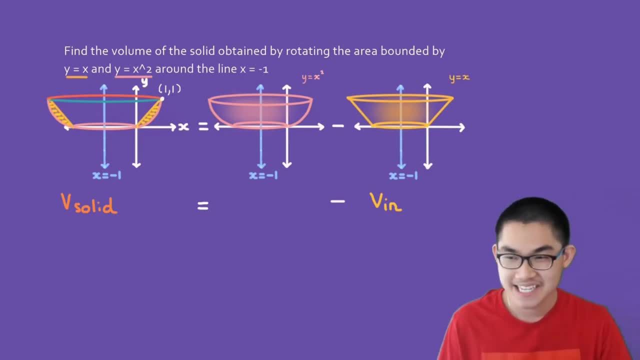 if you remember from the volume formula the formula to find the volume is simply the integral from a to b in that case it's just from 0 to 1 so from here to here which is from 0 to 1 0 to 1 of a of y dy where a of y is the area of the cross section and i'm just going to choose a 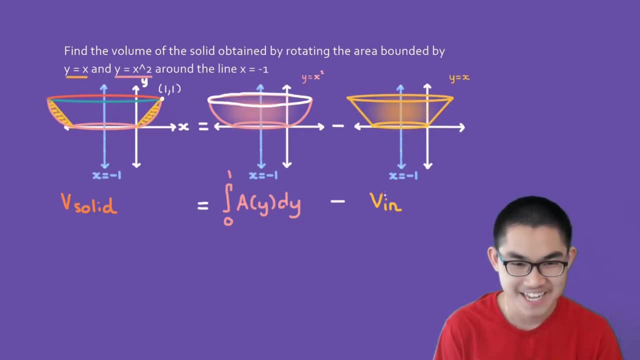 cross section right here so that's our cross section which is a circle now how about the volume of the inner function well it is also the same thing which is the integral from 0 to 1 because from here to here is 0 to 1 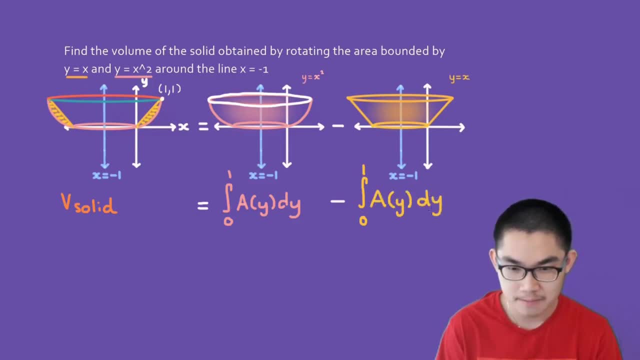 of a of y dy where a of y is going to be the area of the cross section which is a circle 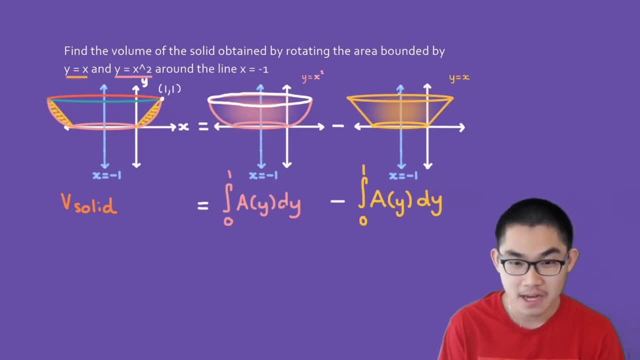 so the next step is to find the area for the cross sections so let's start with the pink one we know 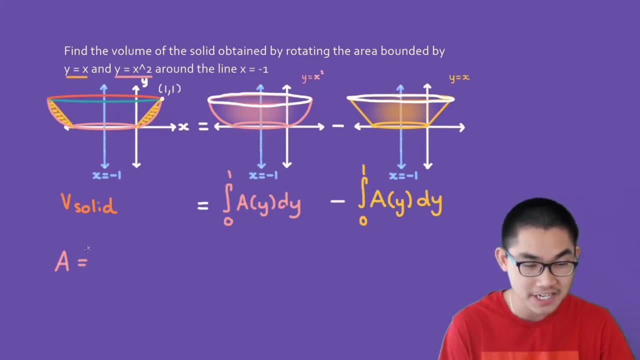 that the area of a circular cross section is going to be pi times the radius to the power of 2. 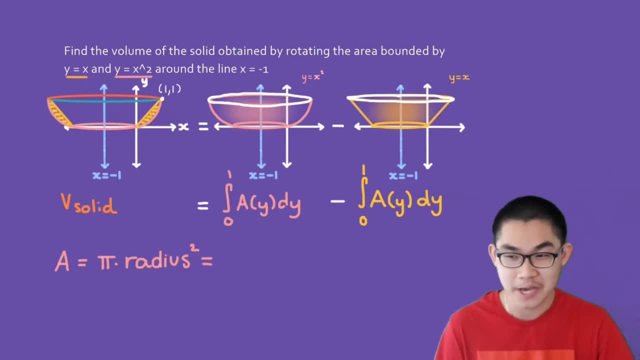 so how do we find the radius well let me show you how to do that so first things first we know that we chose 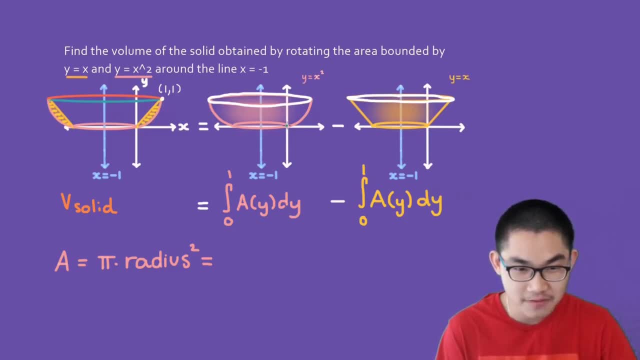 this to be our cross section so the distance from the center until it touches our cross section so 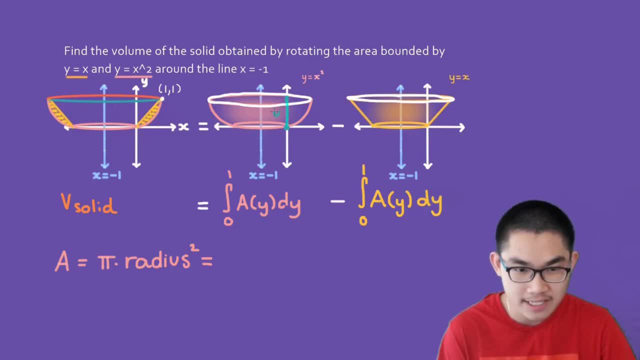 that distance right there is going to be y so that distance is y the distance from the y-axis 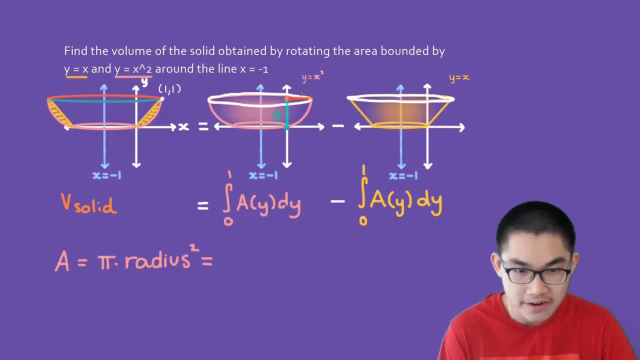 until it touches our function so this distance right here is going to be x and finally since this is negative one 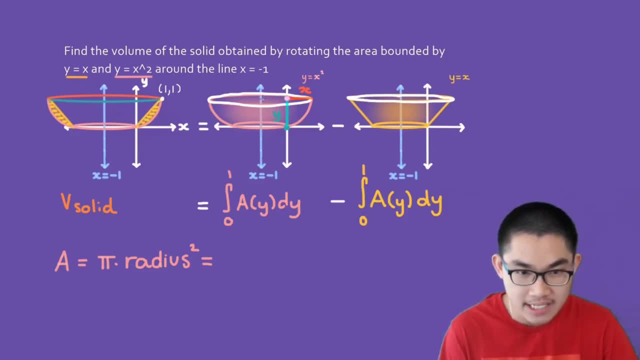 we know that the distance from the y-axis until here that distance is gonna be one 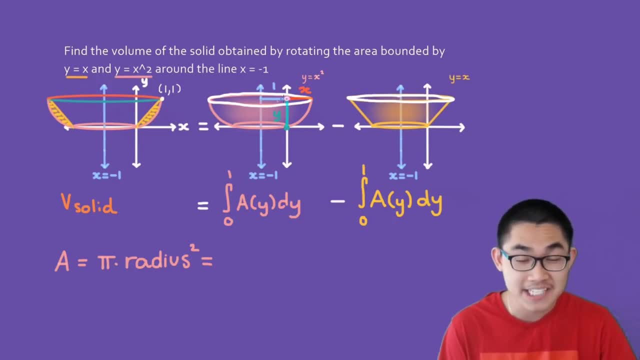 so if you look at the diagram the radius is just x plus one that's it so let's rewrite this this is going to be equal to pi times x plus one to the power of two now there is one formula that you can 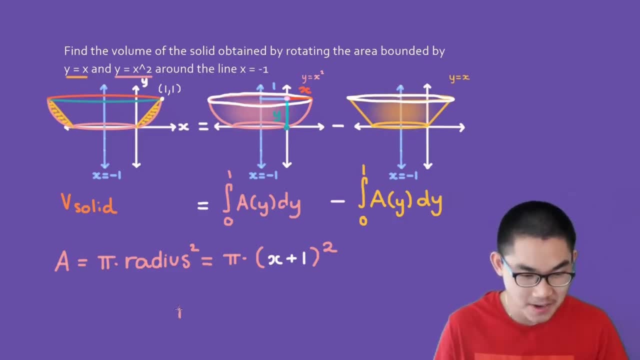 use that will always give you the radius so another thing that we can use is a Velocity Line 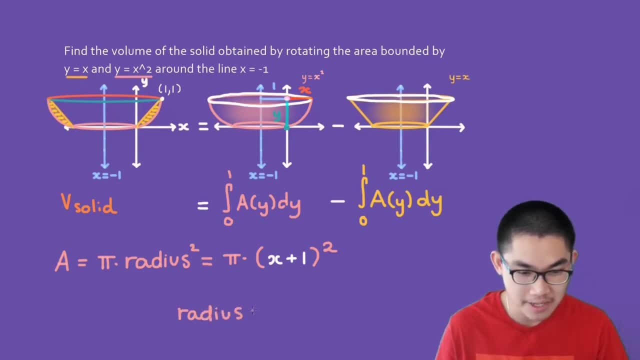 another way to find the radius is to use this formula, which is you take the right x, so take the right x, I'm just going to write x right here, and you minus the left x, so we're going to minus the left x, and the left x is basically this one, so that's going to be minus negative 1, and this formula always works, so take the right x minus the left x, so x minus negative 1 is going to be equal to x plus 1, so that's basically the same as our radius right there. 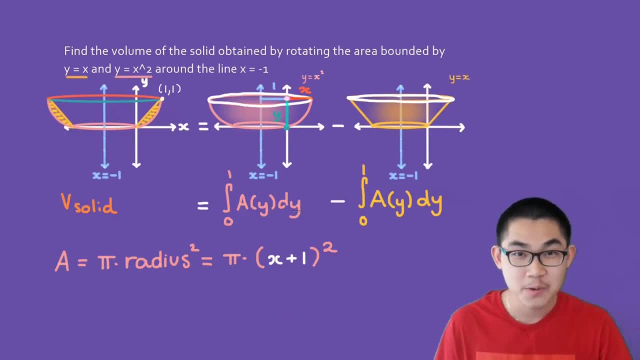 Since we are integrating with respect to y, we have to rewrite our area formula in terms of y, so first things first, we know that the function is y is equal to x to the power of 2, so y is equal to x to the power of 2, which means that x is equal to 1. 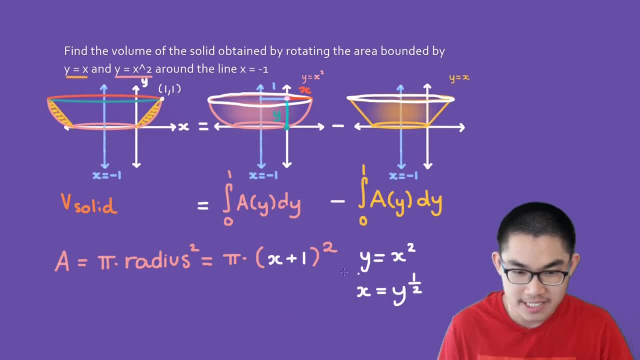 y to the power of 1 half, so let's put this into x right here. So that's going to be y to the power of 1 half plus 1 to the power of 2. So we successfully found the area of our cross-section, and let's put it into our integral. 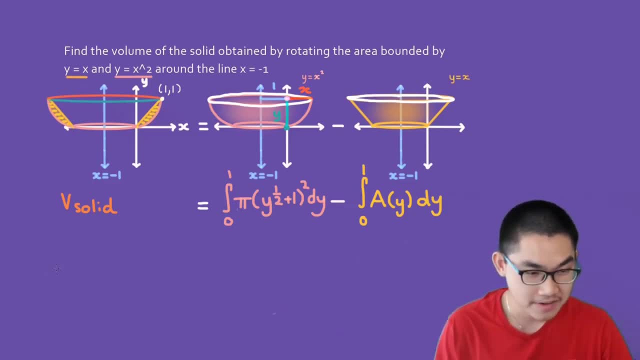 Let's do the same thing for this area right here. So the area, of a circle, is also pi times the radius to the power of 2. 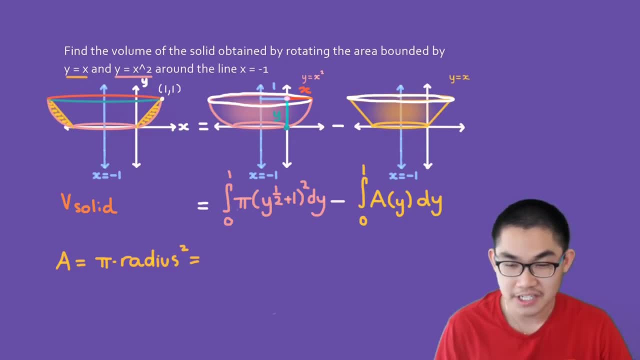 So we chose this to be our cross-section, and we know that the distance from the center until it touches our cross-section, so this distance right there, is going to be y, 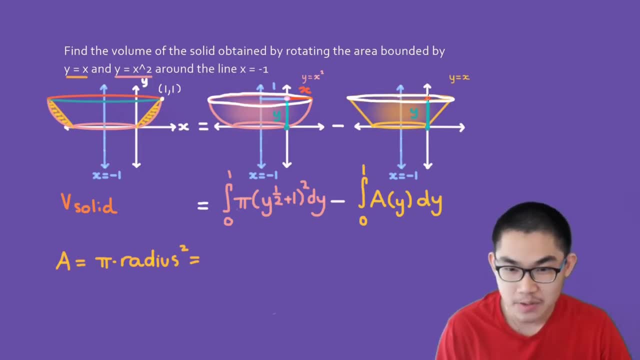 and the distance from the y-axis until it touches our yellow function, so that distance, is going to be x. 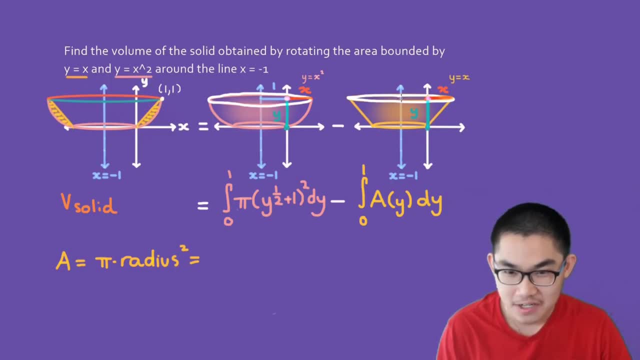 And finally, the distance from here to here, so that distance, is going to be 1. So the radius is just x plus 1. So let's rewrite this. The area is going to be equal to pi times x plus 1 to the power of 2. And since y is equal to x, then we can just rewrite this as pi times y plus 1 divided by 2x to the power of 1. 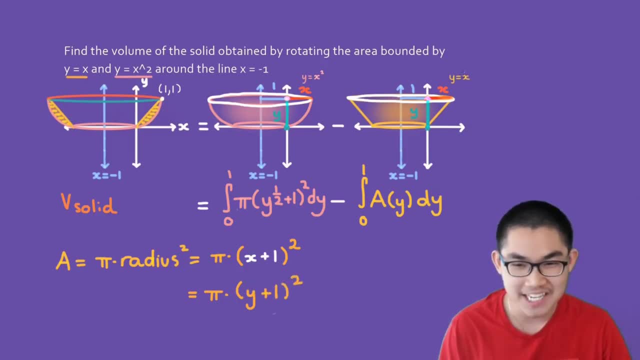 1 to the power of 2 because x is equal to y. So let's put this back into our integral. 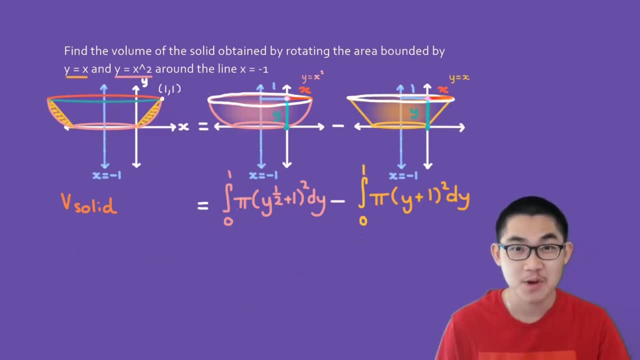 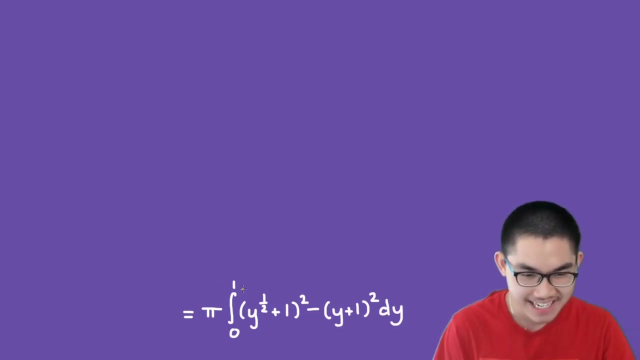 So since both integrals have the same boundaries, we can just match them together into one integral and that's going to make a lot of things easy for us. So this is going to be equal to the integral from 0 to 1 of pi times y to the power of one half plus 1 to the power of 2 minus pi times y plus 1 to the power of 2 dy. So the next step is to factor out the pi's since they are just constants. So let's bring them outside of the integral and we're going to end up with pi times the integral from 0 to 1 of y to the power of 1 half plus 1 to the power of 2 minus y plus 1 to the power of 2 dy. Let's solve for this part right here. So y to the power of 1 half plus 1 to the power of 2 is the same thing as this multiplied by itself. 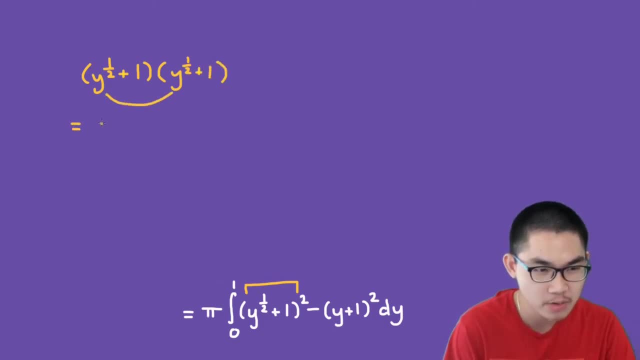 y to the power of 1 half times itself is going to be equal to y. y to the power of 1 half times 1 is going to be y to the power of 1 half and it's the same thing over here. So plus y to the power of 1 half and 1 times 1 is simply going to be 1. So we can rewrite this as y plus 2 times y to the power of 1 half plus 1. And let's put this back into our integral right there. 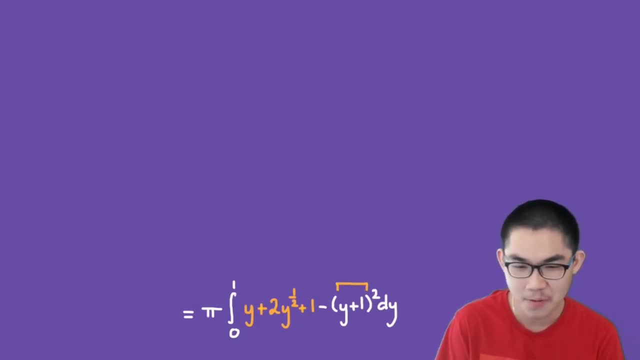 Now how about this part right here? Well, y plus 1 to the power of 2 is the same as y to the power of 2 plus 2y plus 1. So let's put this back into this part right here. Let's keep on going. So this is the same as pi times the integral from 0 to 1 of y plus 2 times y to the power of 1 half plus 1 minus y to the power of 2 minus 2y minus 1. 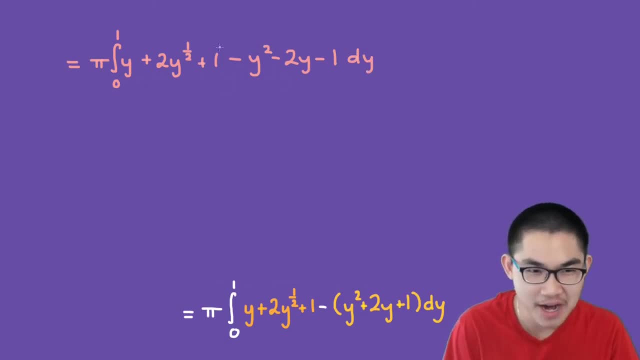 dy. So the first thing we see is that the 1 and the negative ones are going to cancel out. 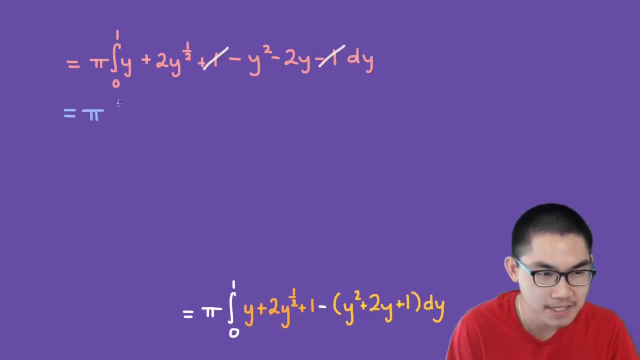 And we're going to have pi times the integral from 0 to 1 of y plus 2 times y to the power of 1 half minus y to the power of 2 minus 2y. And so y minus 2y is going to be negative y. So this is going to be the same. pi times the integral from 0 to 1 of negative y plus 2 times y to the power of 1 half minus y to the power of 2 dy. This is going to be equal to pi times the antiderivative of negative y, which is just negative 1 over 2 times y to the power of 2. Now the antiderivative of 2 times y to the power of 1 half. Now we're going to have y and we plus 1 over here. So that's going to be 3 over 2. We have to divide by that exponent. So we're going to end up with 2 times 2 over 3 times y to the power of 1 half. And if you multiply this, you're going to end up with 4 over 3 times y to the power of 3 over 2. And minus y to the power of 3 over 2. And minus y to the power of 3 over 2. 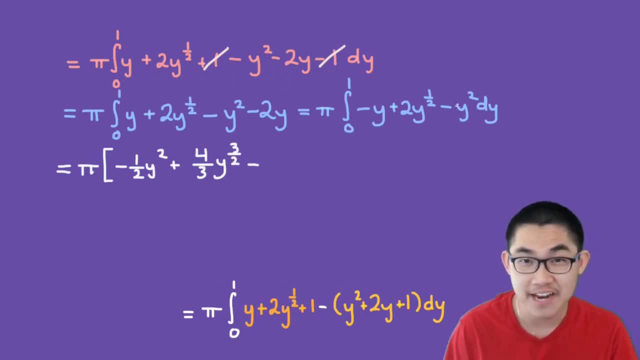 And minus the antiderivative of negative y to the power of 2 is 1 over 3 times y to the power of 3. And the boundary goes from 0 to 1. And we can just go ahead and close that bracket right there. 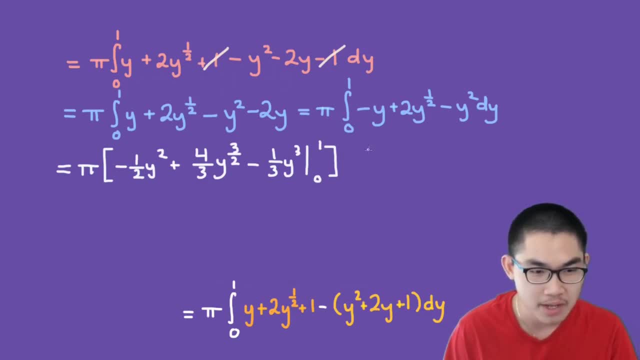 So if you substitute these numbers into our formula, you're going to get pi times negative 1 half plus 4 over 3 minus 1 over 3. Closing the bracket. The next step is just to evaluate these fractions. 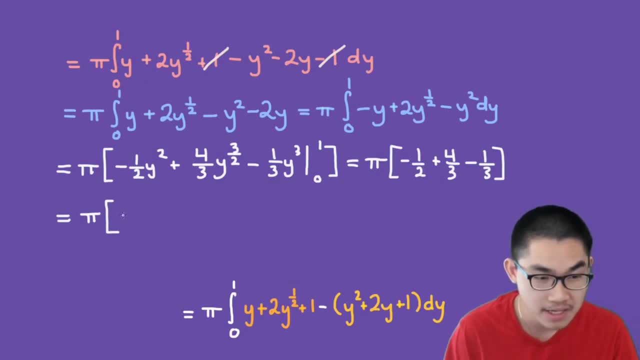 4 over 3 minus 1 over 3 is 3 over 3. And 3 over 3 is just 1, right? So we're going to get 1 over 2 plus 1. And we know that this is the same thing as pi times 1 over 2 positive. 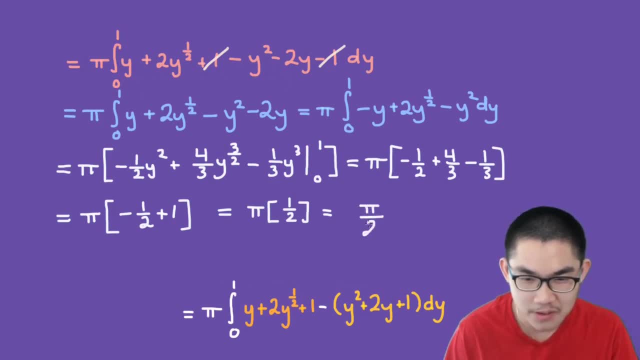 And the final answer is just pi over 2. So this number, let me circle it. So this number right here represents the antiderivative of y to the power of 1 half times y to the power of 3 times y to the power of 2. 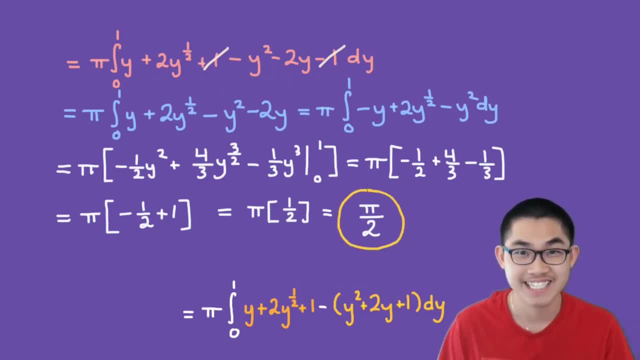 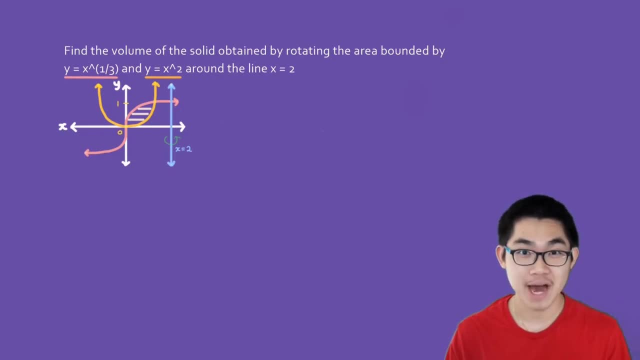 Let's take a look at the particular part of the solution. 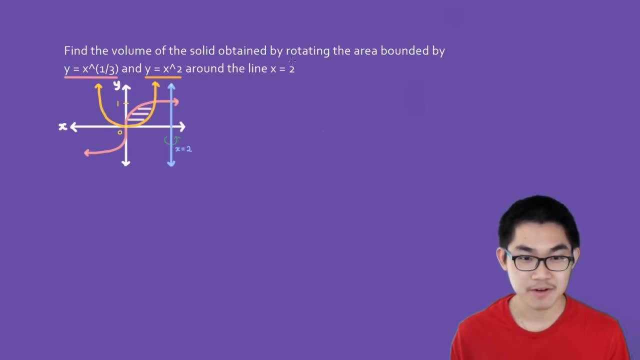 Find the volume of the solid obtained by rotating the area bounded by y is equal to x to the power of one third. That is the pink function right here and y is equal to x square which is the yellow function around the line x is less than x. If we really look at the representation of this area we'd 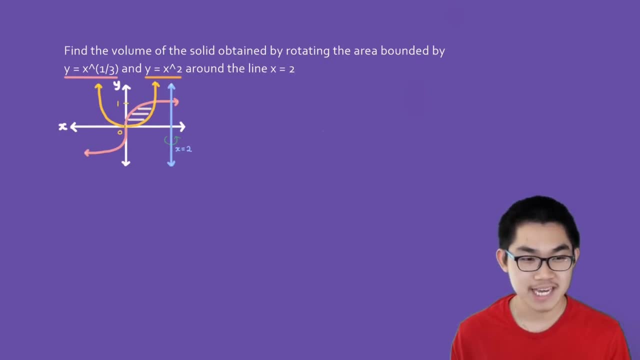 infer that y should be around 1 over 2 plus y, or it should be around 2 thirds of x squared which is low over 3. This sum antibody is taught by 1 over 3 means the routine ofச is equal to 2 so if we take the area between these two functions and we 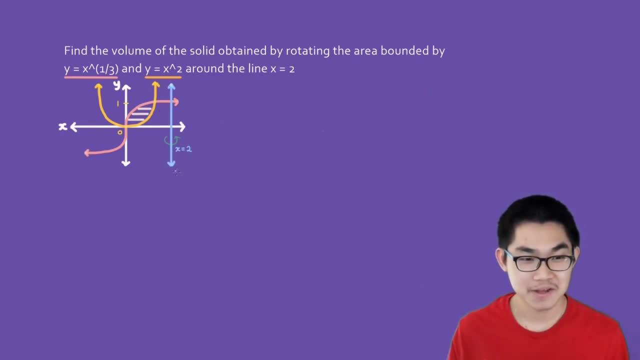 rotate it around the blue vertical line what kind of three-dimensional object are we gonna get well we're gonna get something like this so this is our 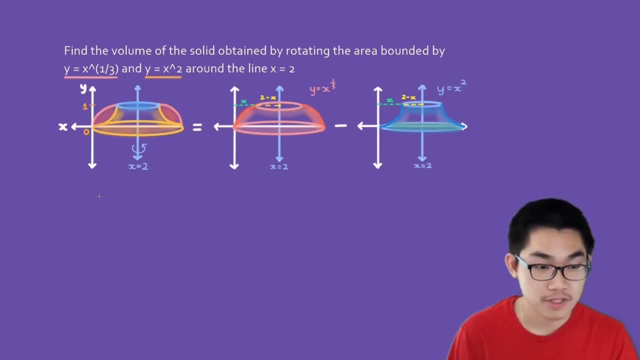 three-dimensional object and we want to find a volume of this object so the volume of this solid so just V solid is equal to the volume of the outside 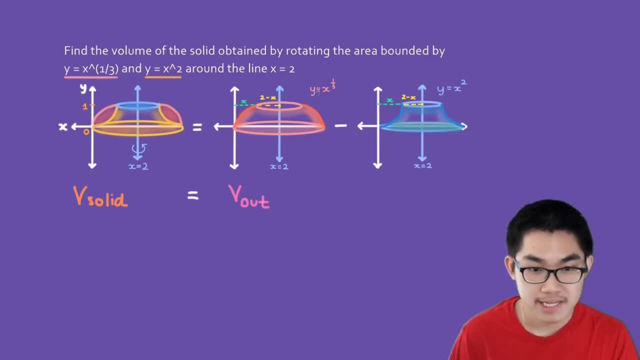 function so the outside function is Y is equal to X to the power of 1 3rd and we don't forget to minus the volume of the inner function so V in where the inner function is Y is equal to X to the power of 2 now if you remember from my previous videos 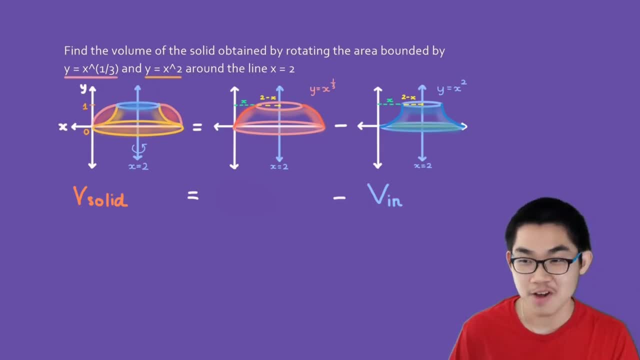 what is the formula to calculate the volume of an object well it's simply the integral from a to B and in this case a to B is just the distance from here to here which is from 0 to 1 so the boundary goes from 0 to 1 of a of y dy where a of y is the area of the cross-section so I'm just gonna take this right here to be the cross-section and we know that this cross-section is a circle or this volume for the volume of the inner function it is the same thing so the integral from 0 to 1 of a of y dy the next step is to find the area formulas so a of y is the same as pi times the radius to the power of 2 because we're trying to find the area of the circular cross-section so what is the radius well we know that the distance from here to here is 2 because this is 0 and that's 2 right so the distance has to be 2 in between and we know that from the center until this distance so this distance where the cross-section is so from here to here is just y and the distance from the y-axis until it touches the function is x so meaning this distance right here is x that's just x so this means 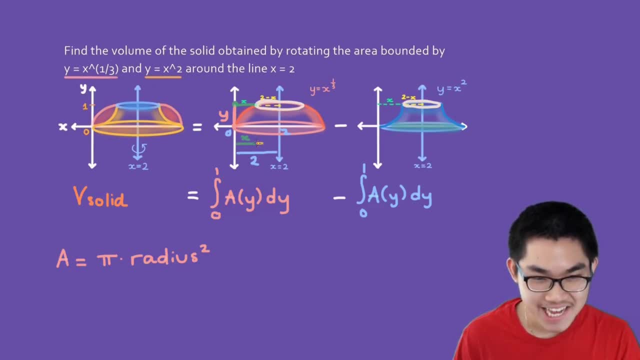 that the radius is right there that's the radius of the circular cross-section and that is simply 2 minus x so this is 2 minus x so let me rewrite this area formula that is just gonna be pi times 2 minus x to the power of 2 so I'm gonna show you a trick the radius you can always find the radius using this formula so just take the right x take the right x which is 2 and minus the left x so the left x is just x right so you just minus x and that's always going to give you the radius you can use a diagram or you can use this formula whichever way you prefer now since we are integrating with respect to y we need to rewrite the area in terms of y so let me show you how to do that now we know that this is y into the object. 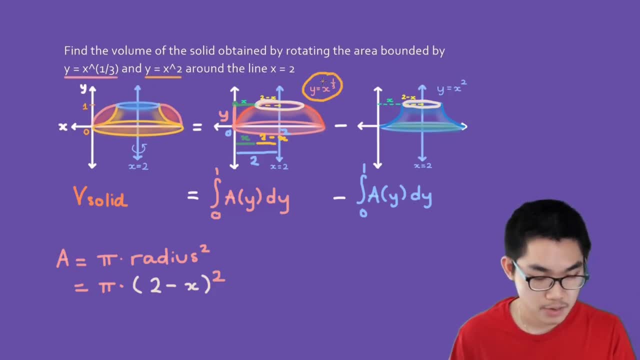 Variable x into the italian. Now we know that the grper angle is from the y-axis towards the space between to the being point we need to rewrite the area in terms of y so let me show you how to do that now we know that this is y taken a little it is 2 minus the Forward 2 pi times theえ and the allies 1 times primary feet x. know that this function is y is equal to x to the power of one third so y is equal to x to the power of one third which means that x is equal to y to the power of three you just take both sides to the power of three and this is what you get so the area is the same as pi times two minus y to the power of three and this whole thing to the power of two and we're ready to put this back into our integral let's do the same thing over here so the area is also pi times the radius to the power of two because that's the area for a circular cross-section and since we pick the cross-section to be here then distance from the center until we reach the cross section is y we also know that the distance from the y-axis until it touches the function is x we can call that distance x and the distance from here until it reaches the vertical line or we can just do it like this so the distance from here here is two so if you take a look at this diagram the radius which is this distance is just 2 minus x so let's put it back into our area formula so the area is equal to pi times two minus x to the power of 2. now since we are integrating with respect to y we have to rewrite this 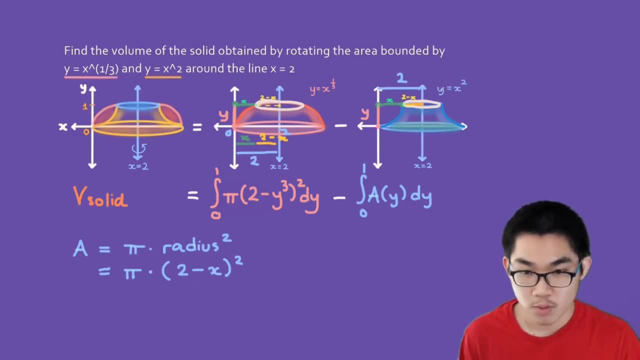 function in terms of y so we know that this is y-axis then we also know that this is y-axis equal to x to the power of 2. so here is y equal to x to the power of 2 and this means that x is 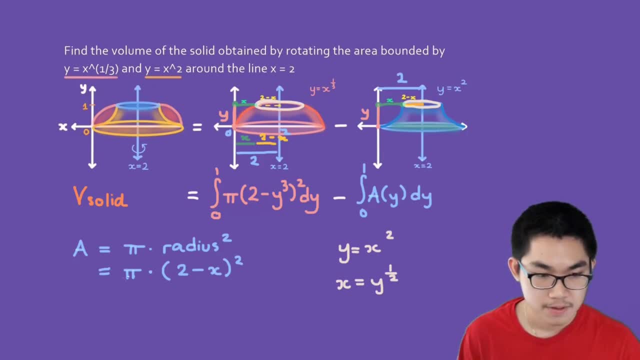 equal to y to the power of 1 half so this is the same as pi times 2 minus y to the power of 1 half 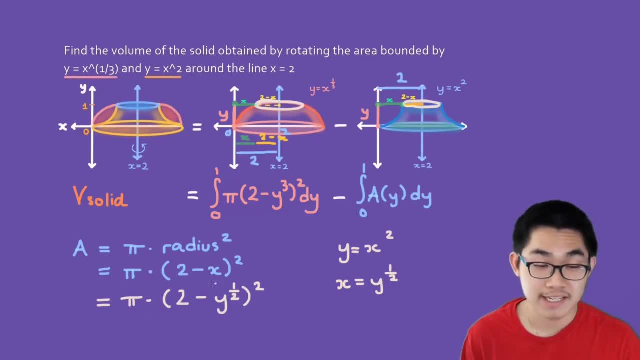 to the power of 2 and so we successfully rewrite this in terms of y let's put it back into our integral now since both of these integrals have the same boundaries we can just smash them together 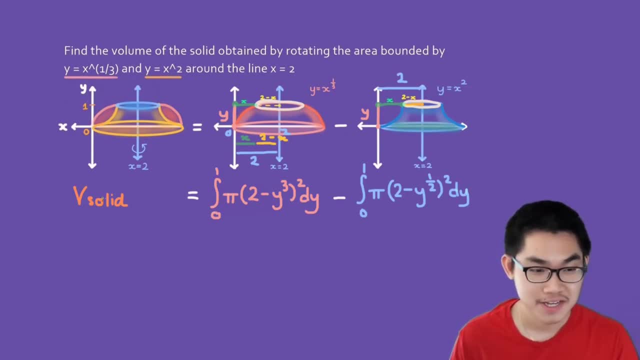 into one integral and that's going to simplify a lot of things so the volume of the solid is equal to the integral from 0 to 1 of pi times 2 minus y to the power of 3 to the power of 2 minus i times 2 minus y to the power of 1 half to the power of 2 dy. And the next step is to factor out the pi. 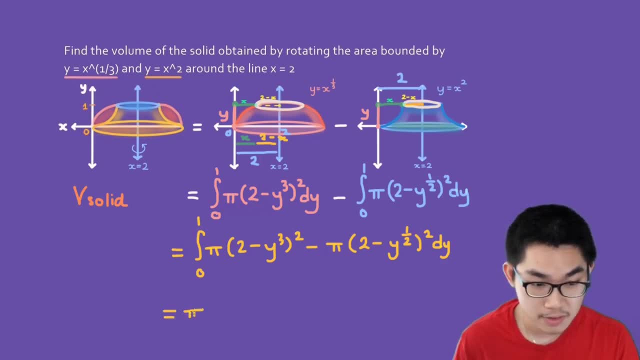 So since pi is just a number, we can just bring it outside of the integral. So this is the same 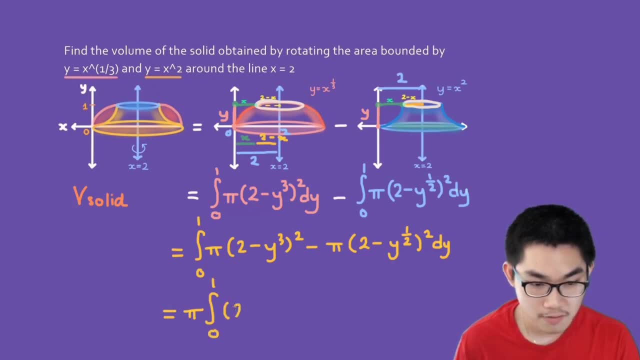 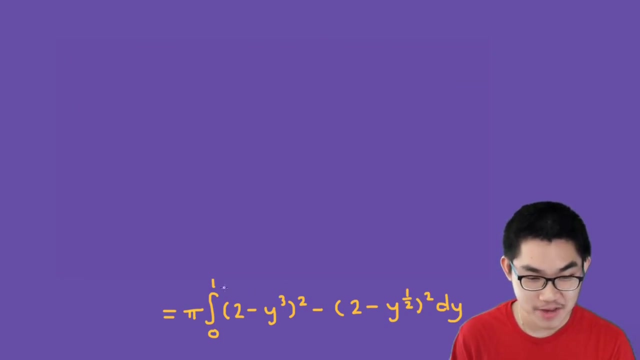 as pi times the integral from 0 to 1 of 2 minus y to the power of 3 to the power of 2 minus 2 minus y to the power of 1 half to the power of 2 dy. Now, looking at this, the first thing we have to do is solve for this. So 2 minus y to the power of 3 to the power of 2 is the same as 2 minus y to the power of 3 times itself. Now, 2 times 2 is going to be 4. 2 times negative y to the power of 3 is negative. negative 2 times y to the power of 3. It's the same thing here. So minus 2 times y to the power of 3. And negative y to the power of 3 times itself is positive y to the power of 6. So let's just put it like this. Let's just put it as y to the power of 6 minus 4 times y to the power of 3 plus 4. So let's put this back into our integral. 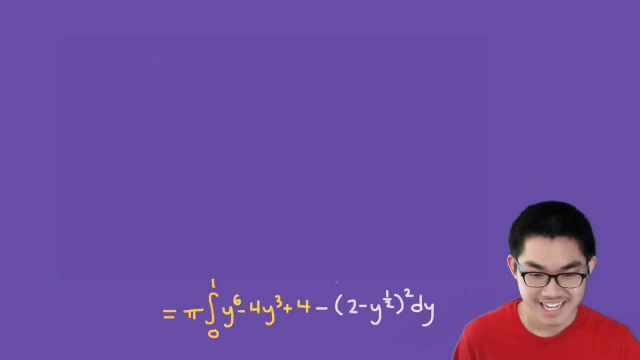 So let's do the same thing for this one right there. So this is the same as 2 minus y to the power of 1 half times itself. Now 2 times 2 is going to be 4. 2 times negative y to the power of 1 half is negative 2 times y to the power of 1 half. And this right here is going to be the same. So minus 2 times y to the power of 1 half is negative 2 times y to the power of 1 half. And negative y to the power of 1 half times itself is just positive y. And so this is the same as y minus 4 times y to the power of 1 half plus 4. And let's put this back into this part right here. So let's keep on going. This right here is the same as i times the integral from 0 to the power of 1 half. And so this is the same as y minus 4 times y to the power of 1 half. And so this is the same as i times the integral from 0 to 1 of y to the power of 6 minus 4 times y to the power of 3 plus 4 minus y plus 4 times y to the power of 1 half minus 4 dy. 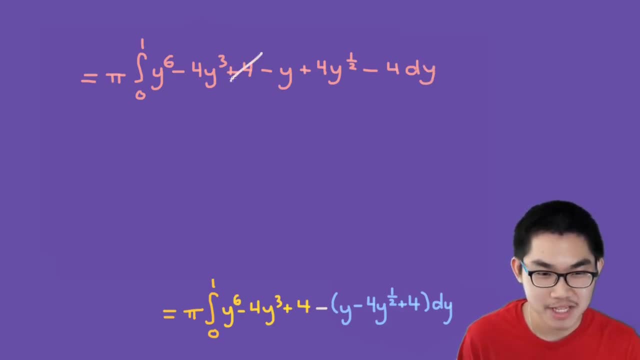 And so if you look here, 4 minus 4 will just cancel themselves out. 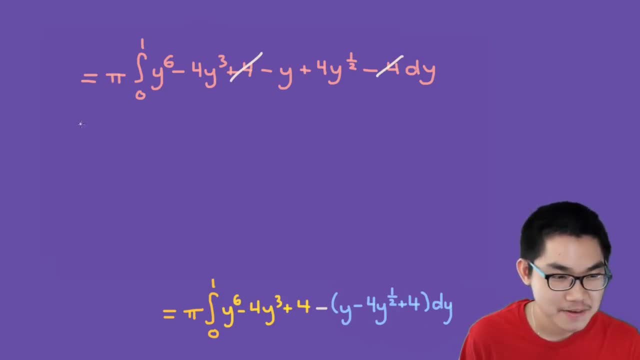 And so this is the same as i times the integral from 0 to 1 of y to the power of 6 minus 4 times y to the power of 3 minus y plus 4 times y to the power of 1 half dy. This is the same as pi times the antiderivative of y to the power of 1 6 which is just 1 over 7 times y to the power 7. For this one the antiderivative of this is just 4 times y to the power of 4 and you divide by 4 so you're just gonna get y to the power of 4 and for negative y you're just gonna get 1 over 2 times y to the power of 2. For this one you're gonna get 4 times y to the power of 3 over 2 and you divide it by 3 over 2 so what you're gonna get is 4 times 2 over 3 times y to the power of 3.